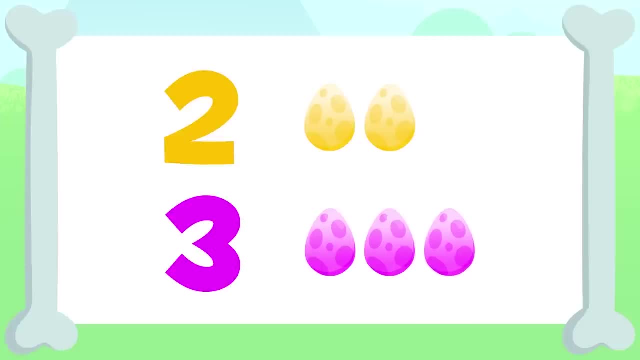 And down there we have one, two and three eggs. We have to add two plus three, So all the eggs together would sum up one, two, three, four and five. We have five eggs. Two plus three equals five. The result of adding up two plus three is five. Well done, Dino Do. 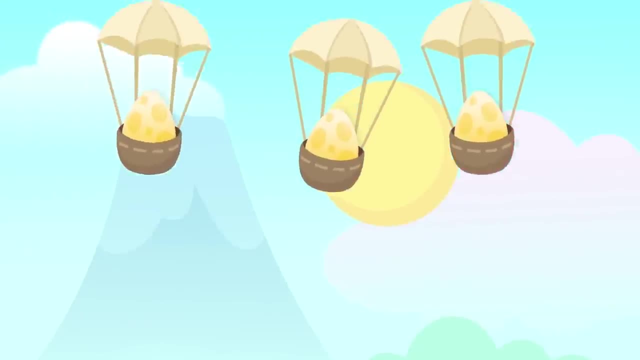 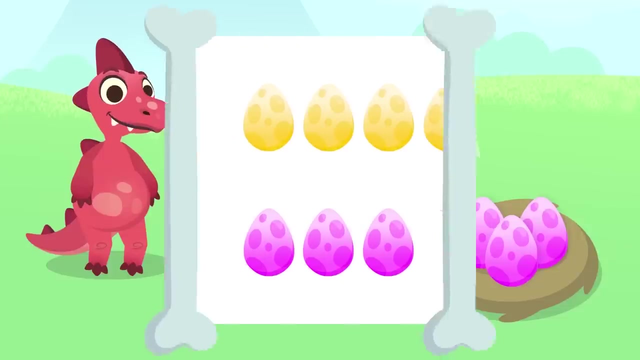 you like adding up. Whoa more eggs are falling down. Let's add them up to find out how many eggs in total you'll have to look after. okay, Up here there are one, two, three, four and five eggs. 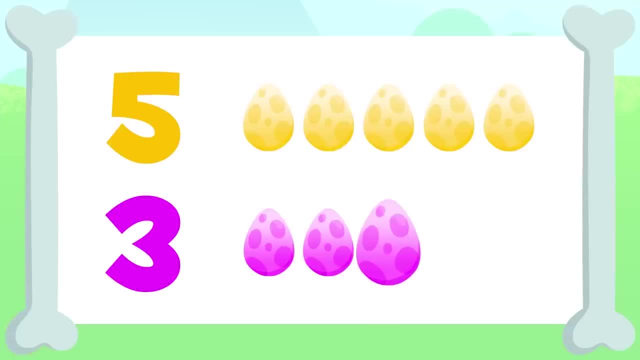 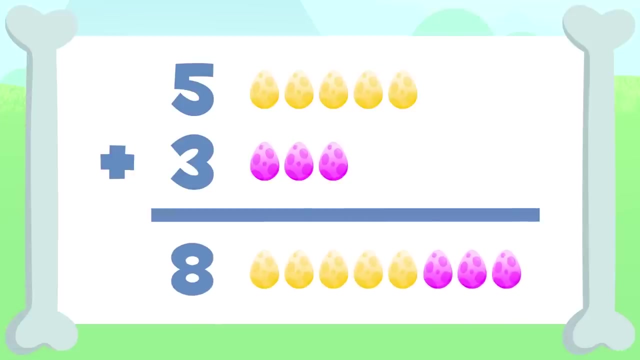 And down there we have one, two and three eggs. We have to add five plus three. So the result of adding up is five plus three. So all the eggs together would sum up one, two, three, four and five. We have eight. Five plus three equals eight. Well done, Dino Today. 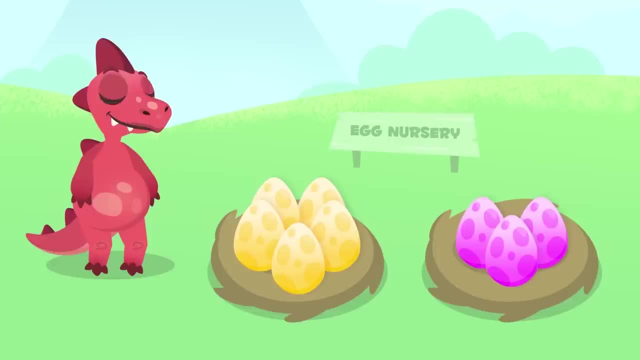 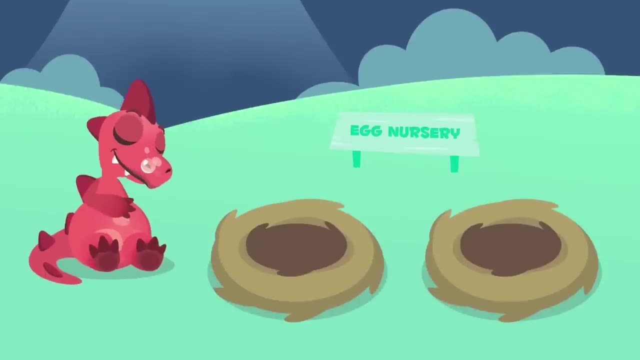 you need to look after eight dinosaur eggs. Now you know how to add up What: One, two, three, four and five. Oh, I'm going to add nine. Oh, You've fallen asleep again. Dino, Wake up. Everyone's gone. You're not much of a dinosaur. 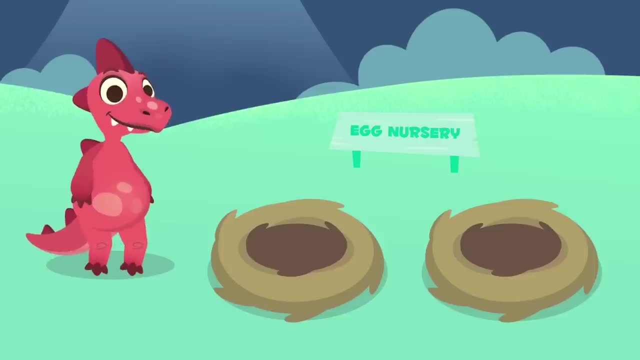 egg guardian, are you? No, No, No. Well, it's okay, Don't think too much about it, Just sleep, Sleep, Sleep, Sleep. Well, it's okay, Dino, Today we've learned how to add. 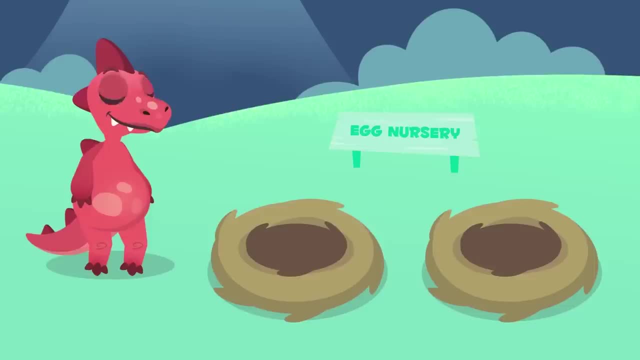 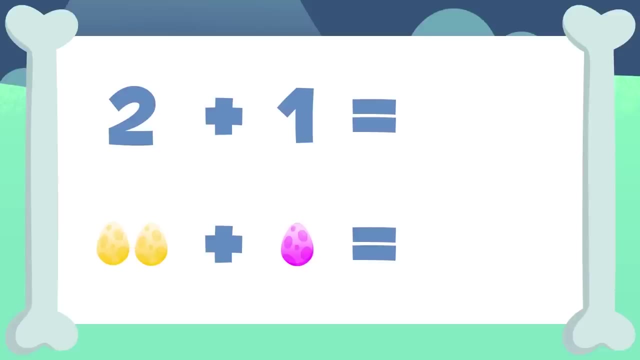 Do you want to recap? We could also do horizontal additions. It's done in the same way. Pay attention: Two plus one equals one, two and three. Two plus one equals three. Very well, Let's do the next one. 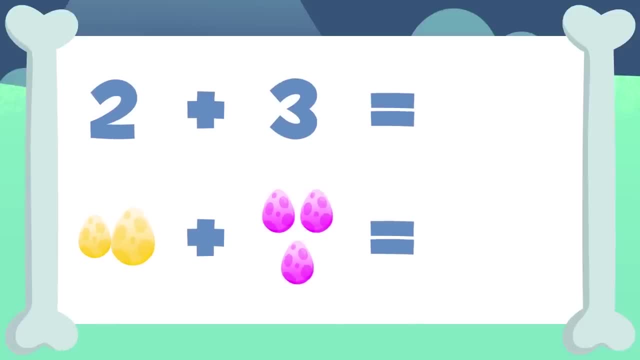 Two plus three equals one, two, three, four and five. Two plus three equals five. Way to go, Let's do another. one. Five plus three equals one, two, three, four, five, six, seven and eight. 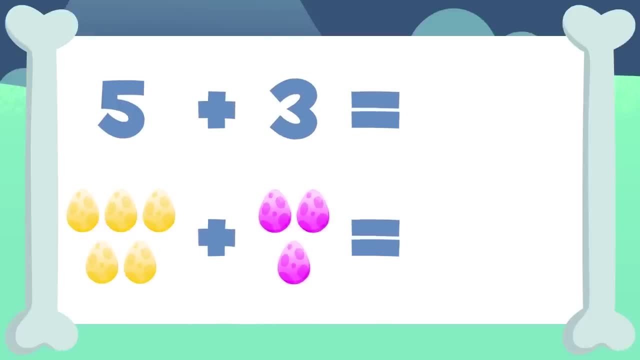 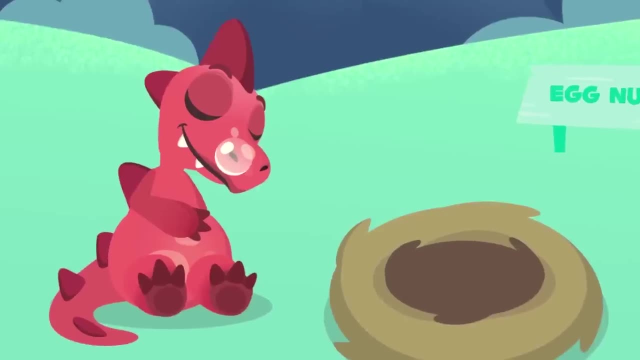 Five plus three equals eight. So good. I'm afraid there's nothing we can do about Dino. He's had a hard day, so we'll just let him sleep a bit more. See you around, Dino, Bye. See you around everyone. 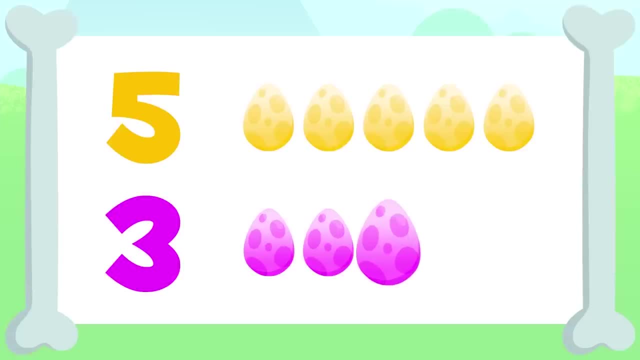 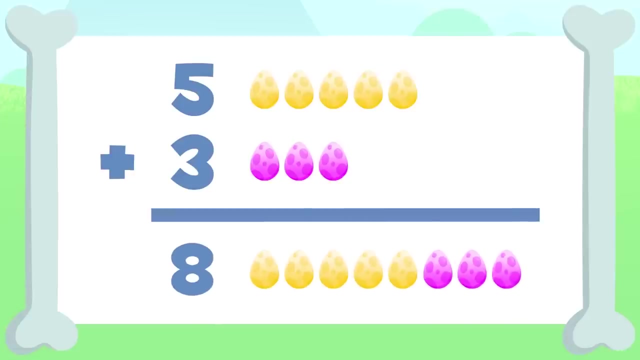 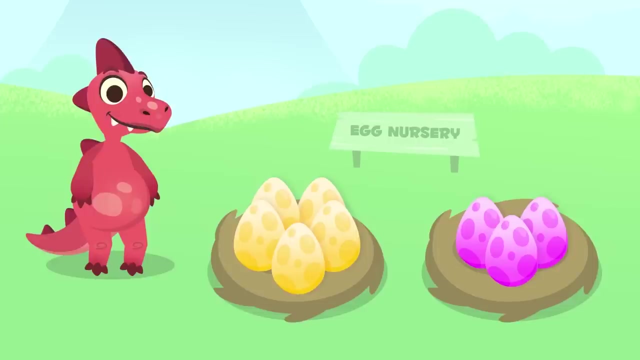 And down there we have one, two and three eggs. We have to add five plus three. So the result of adding up two plus three is five. So the result of adding up two plus three is eight. Well done, Dino. Today you need to look after eight dinosaur eggs. Now you know. 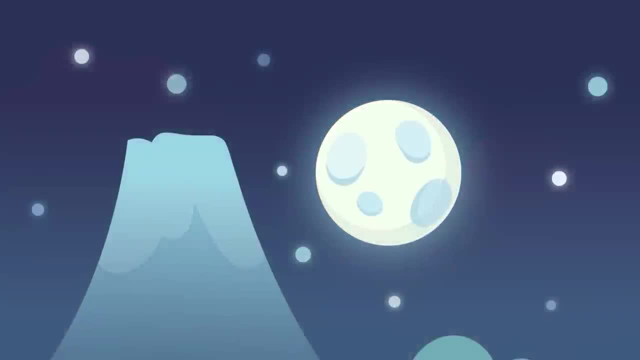 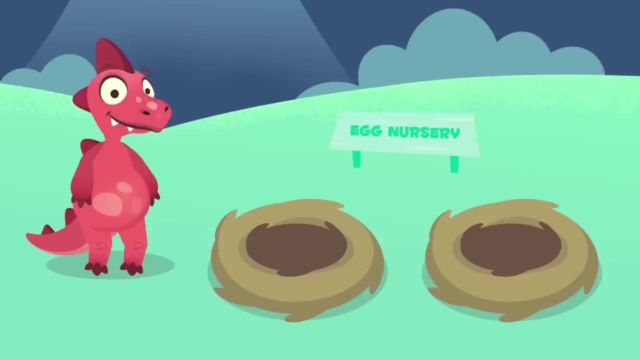 how to add up. You've fallen asleep again, Dino. Wake up. Everyone's gone. You're not much of a dinosaur egg guardian, are you? Well…it's okay, Dino know, today we've learned how to add. do you want to recap? we could also do horizontal additions. 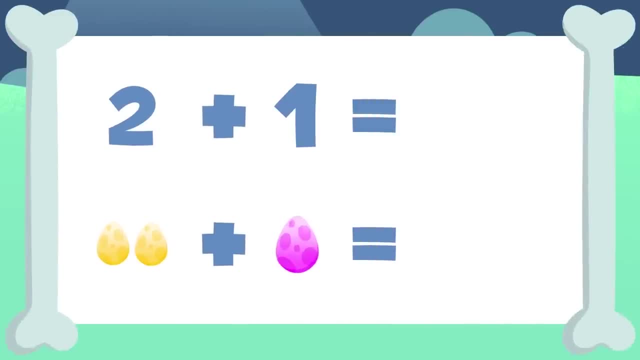 it's done in the same way. pay attention: two plus one equals one, two and three. two plus one equals three. very well, let's do the next one. two plus three equals one, two, three, four and five. two plus three equals five. way to go, let's do another one. five plus three equals one, two, three. 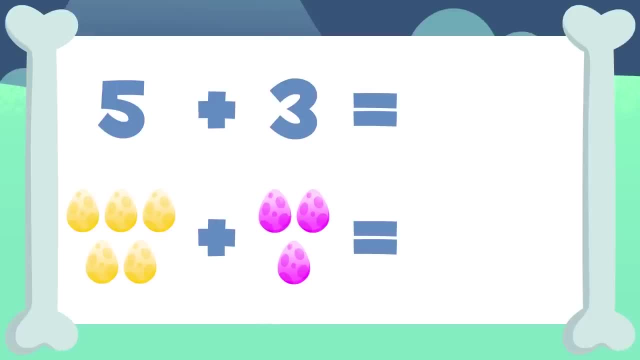 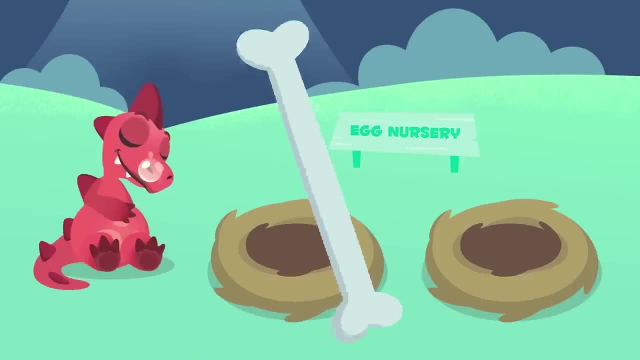 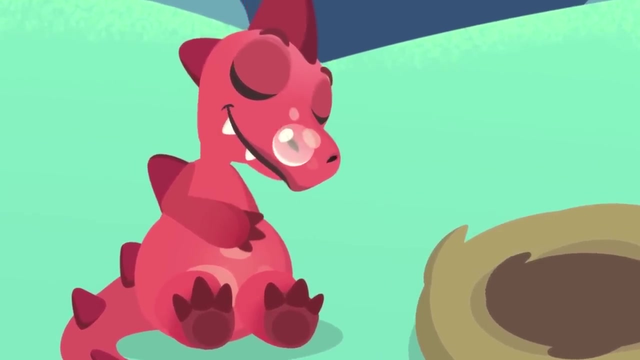 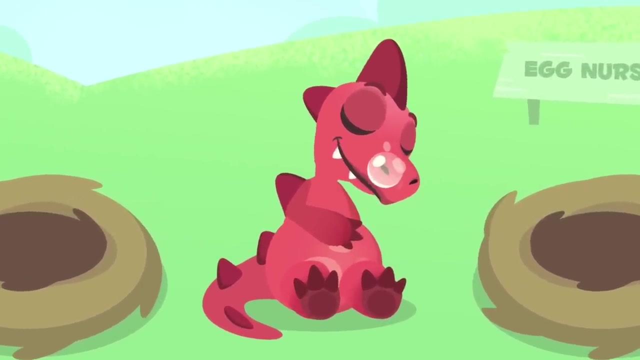 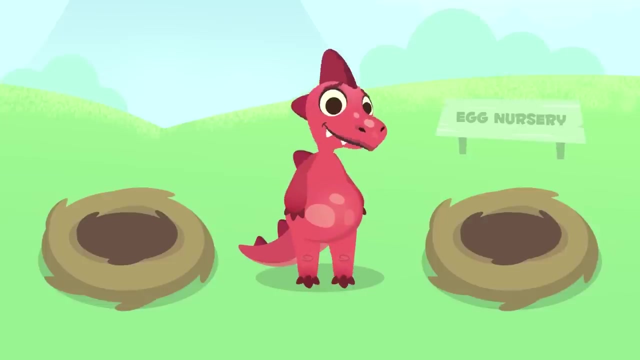 four, five, six, seven and eight. five plus three equals eight. so good, I'm afraid there's nothing we can do about dino. he's had a hard day, so we'll just let him sleep a bit more. see you around everyone. hey, dino, you fell asleep again. my, my, I see you're not doing much. are you bored? let's go get some. 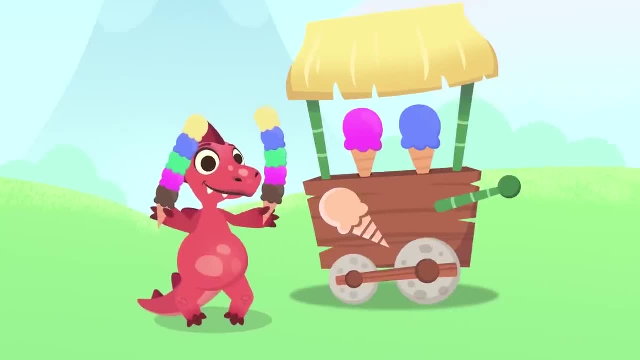 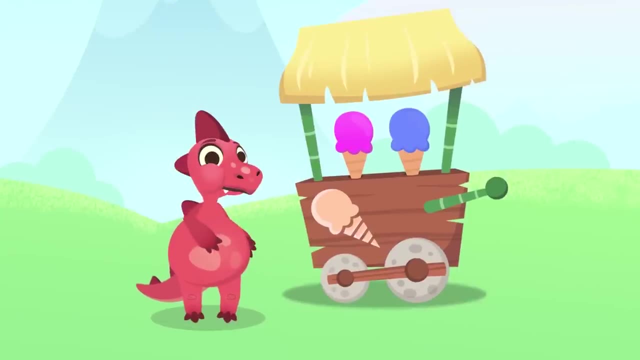 ice cream. whoa dino, you got yourself two huge ice creams. it'll take you long to eat them both. wow, you were really hungry, weren't you? now that we're full, we can practice additions. what do you say? Come on, let's add. How many ice creams are there? 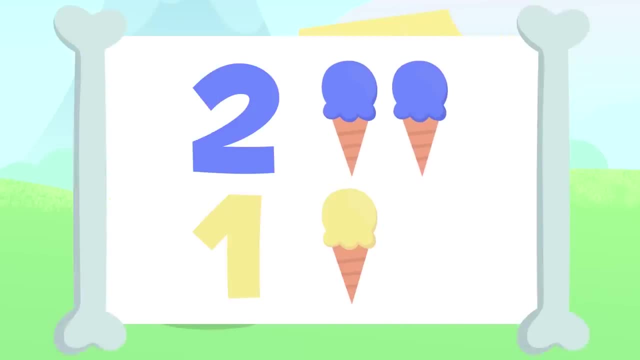 Up here we have one and two And down there we have one. Go ahead, you do the adding. I'll give you a few seconds. You got it. Let me try All ice creams together would be one, two, three. 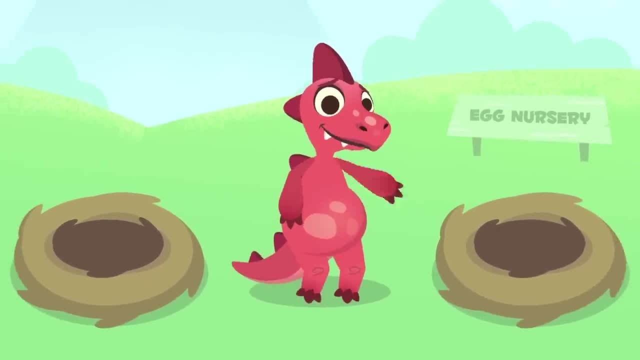 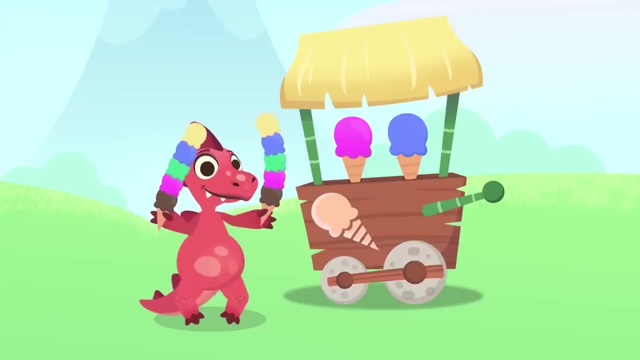 Hey, Dino, You fell asleep again. My my, I see you're not doing much. Are you bored? Let's go get some ice cream. Whoa Dino, You got yourself two huge ice creams. It'll take you long to eat them both. 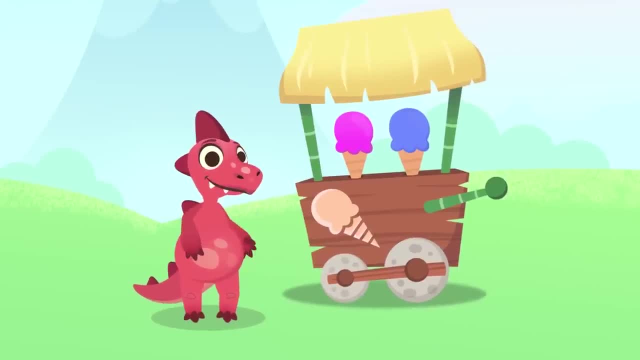 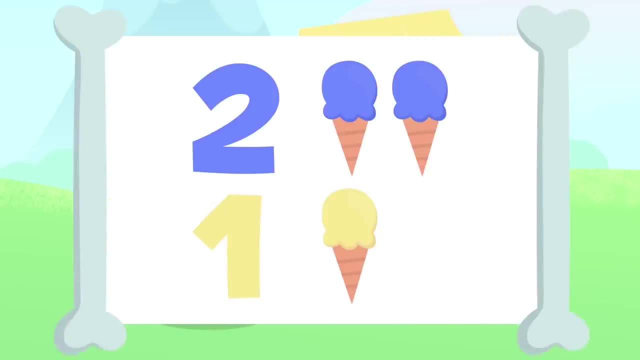 Wow, you were really hungry, weren't you? Now that we're full, we can practice additions. What do you say? Come on, let's add. How many ice creams are there? Up here we have one and two, And down there we have one. 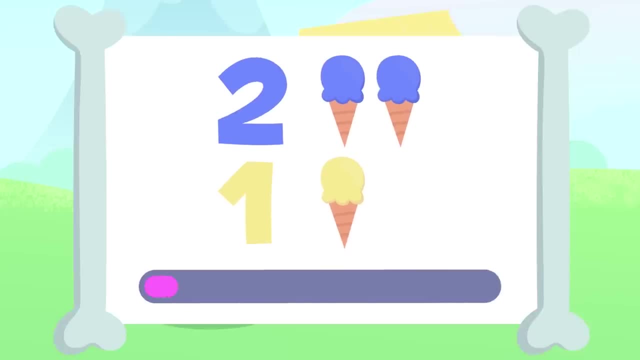 Go ahead. You do the adding. I'll give you a few seconds. You got it. Let me try. All ice creams together would be one, two, three, four, five, six, seven, eight. You got it: One, two, three. 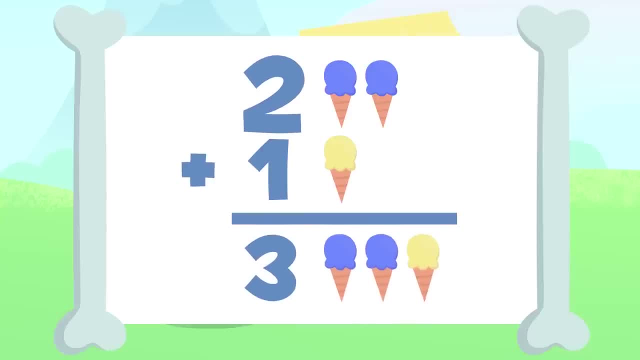 Three. There are three ice creams. Two plus one equals three. We just did our first addition. The result of adding two plus one is equal to three. Well done, Dino, Let's try another one. There's one ice cream up here and three down there. 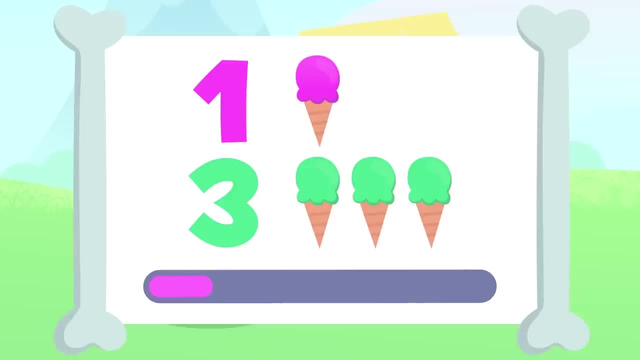 Why don't you add them up? Take your time, You got it. If we add these ice creams together, we'll have in total one, two, three and four. Four. We have four ice creams in total. One plus three equals four. 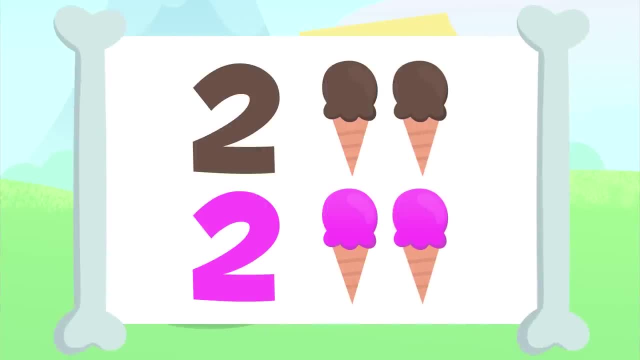 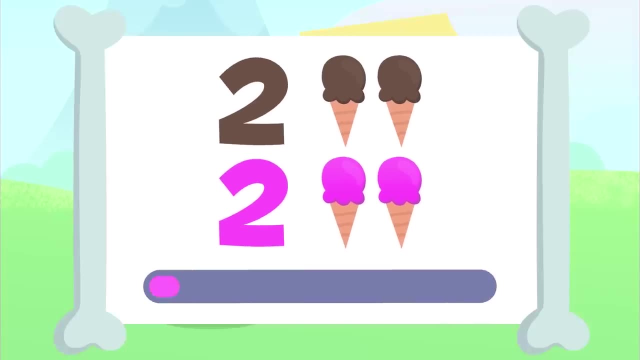 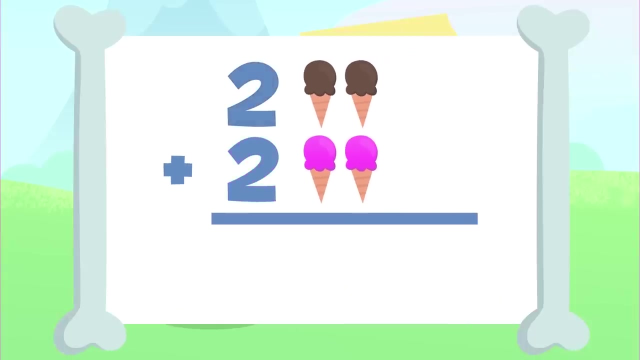 Shall we carry on Now? you'll have to add these two ice creams up here to those two ice creams down there. I'll give you a few seconds to add them up. How did that go? You got it. The result of adding up two plus two is one, two, three and four. 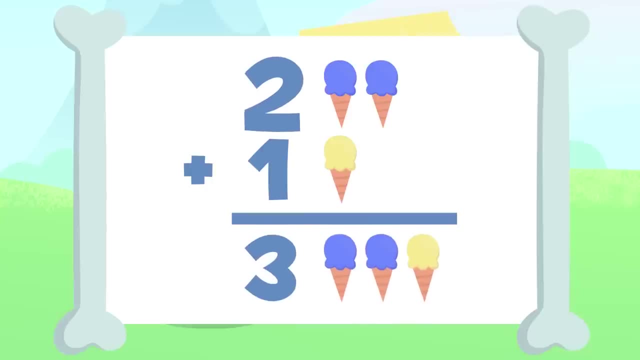 Three. there are three ice creams. Two plus one equals three. We just did our first addition. The result of adding two plus one is equal to three. Well done, Dino, Let's try another one. There's one ice cream up here and three down there. 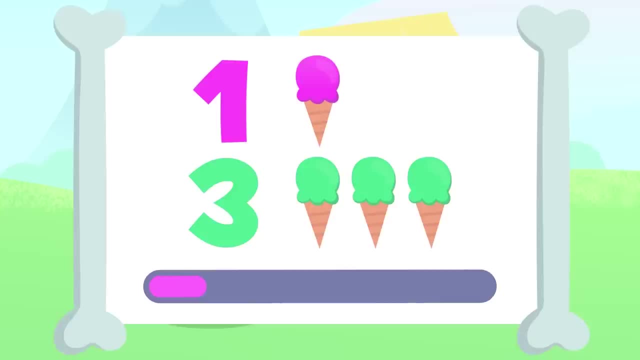 Why don't you add them up? Take your time, You got it. If we add these ice creams together, we'll have in total one, two, three and four. Four, Four. We have four ice creams in total. One plus three equals four. 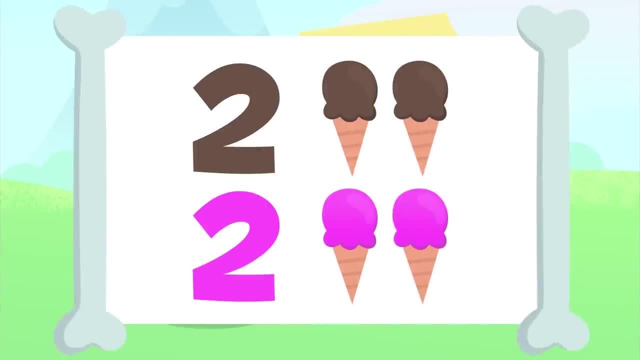 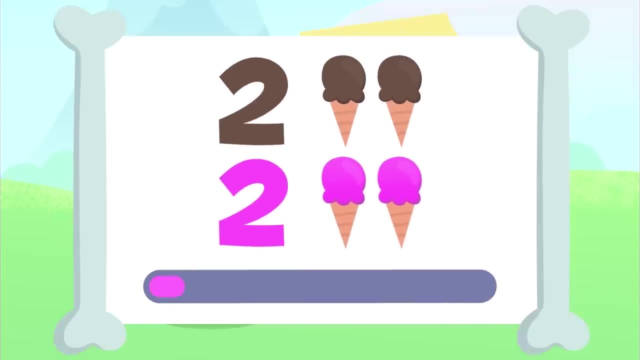 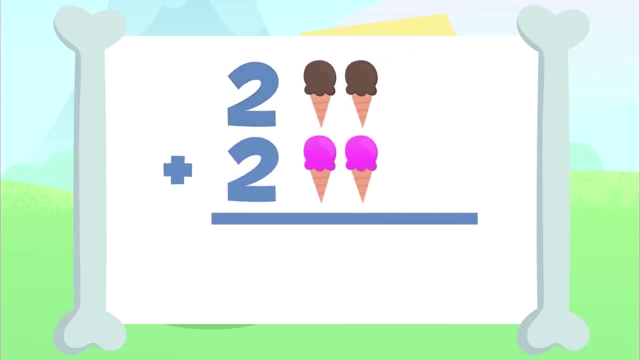 Shall we carry on? Now? you'll have to add these two ice creams up here to those two ice creams down there. I'll give you a few seconds to add them up. How did that go? You got it. The results of adding up two plus two is one, two, three and four. 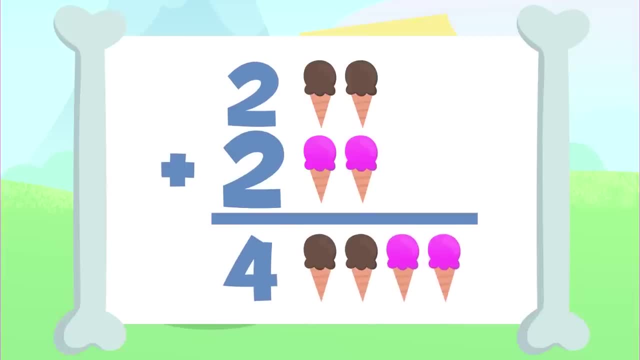 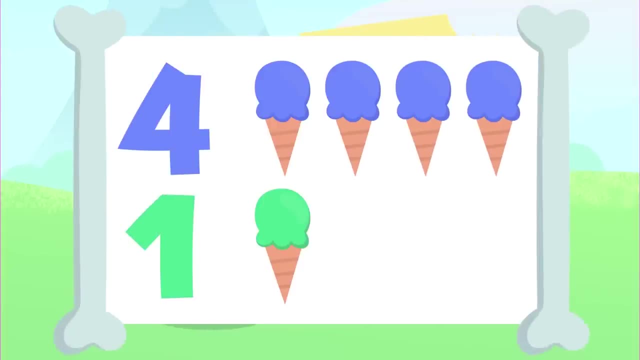 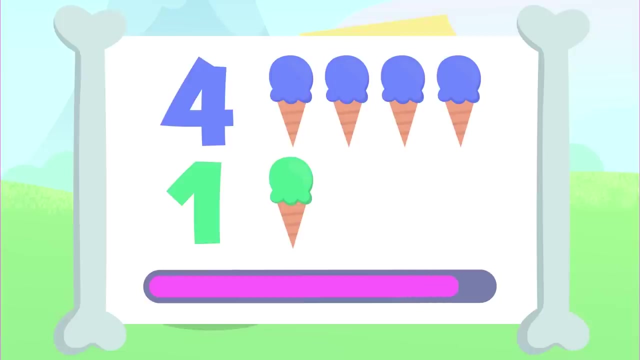 Four. There are four ice creams. Two plus two equals four. Let's try another one. You'll have to add these four ice creams up here To the one ice cream cream down there. Let's go for it. You got it. The result of adding up 4 plus 1 is 1,, 2,, 3, 4,. 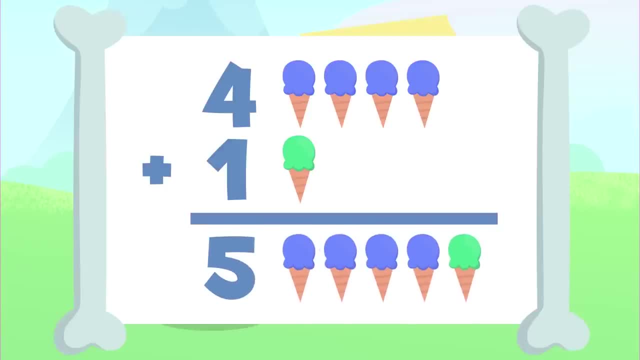 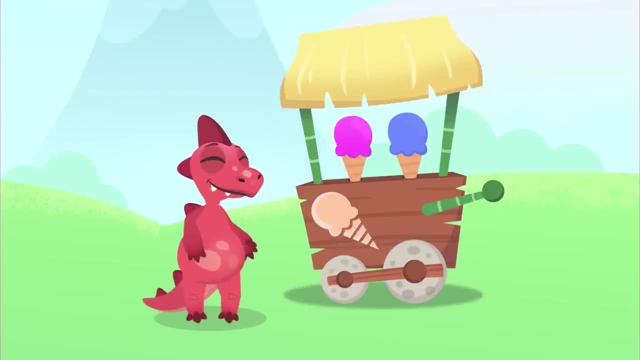 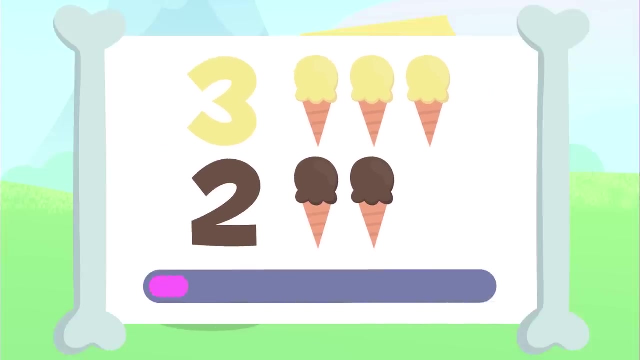 and 5.. 5!, There are 5 ice creams. 4 plus 1 equals 5.. Shall we try the last one? We have to add these 3 ice creams up here to those 2 ice creams down there. Let's go for it. That's it, The result of. 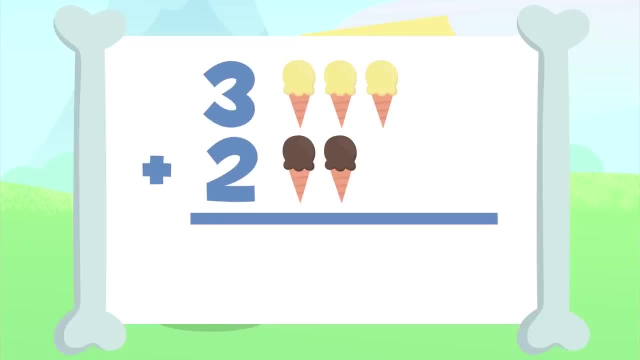 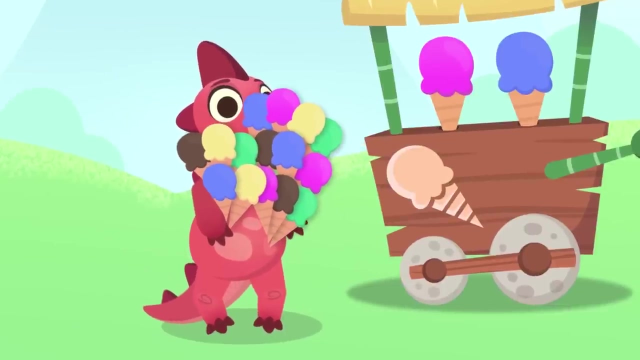 adding up 3 plus 2 is 1,, 2,, 3,, 4, and 5.. 5!, There are 5 ice creams. 3 plus 2 equals 5.. And what are you going to do with all this ice cream Dino? Are you going to eat it? 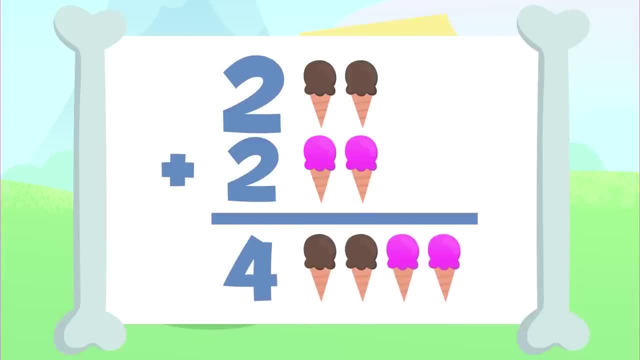 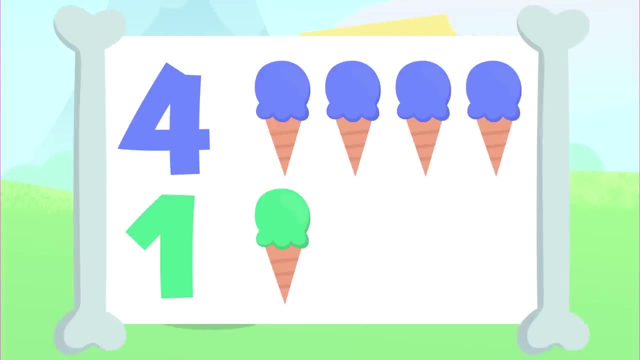 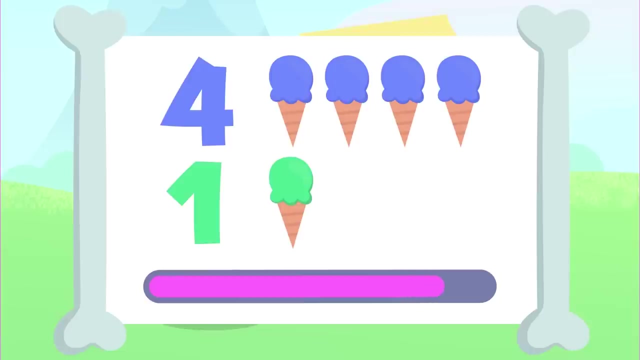 Four. There are four ice creams. Two plus two equals four. Let's try another one. You'll have to add these four ice creams up here to the one ice cream down there. Let's go for it. You got it. The result of adding up four plus one is one, two, three, four and five. 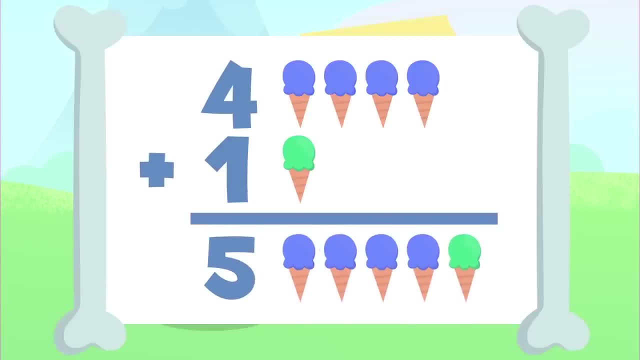 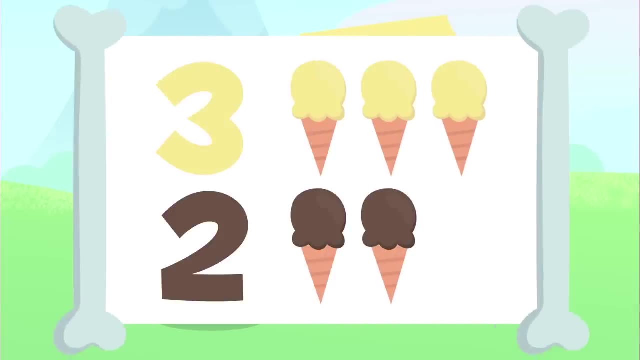 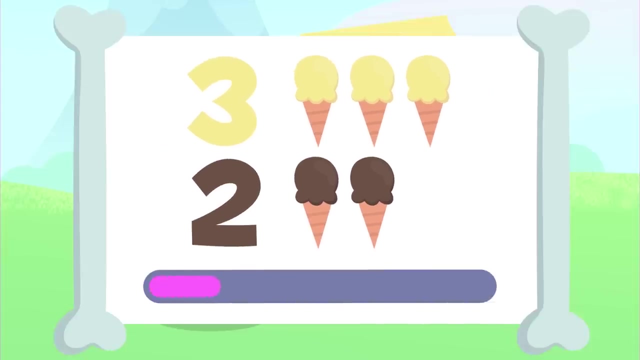 Five. There are five ice creams. Four plus one equals five. Shall we try the last one? We have to add these three ice creams up here to those two ice creams down there. Let's go for it. That's it. The result of adding up three plus two is one, two, three and four. 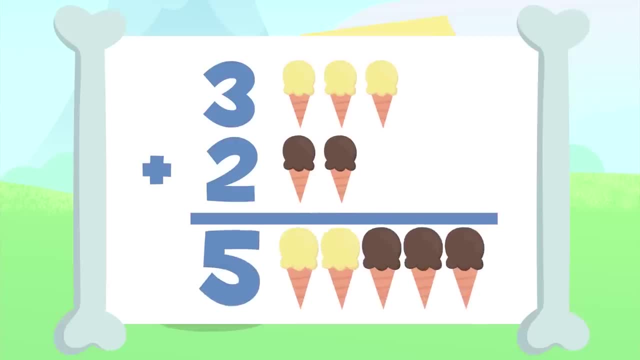 Three, four and five, Five. There are five ice creams. Three plus two equals five. And what are you going to do with all this ice cream, Dino? Are you going to eat it? You're going to feel sick, Dino. 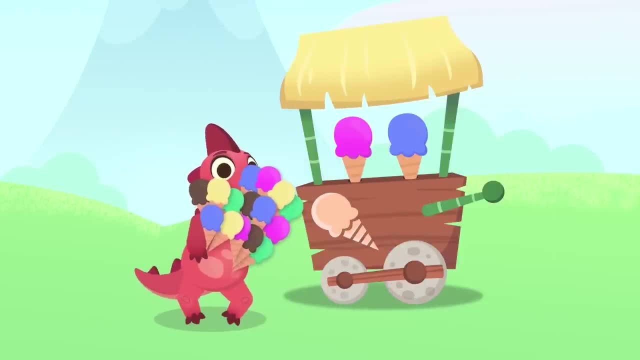 Wouldn't it be best if you save it for later? My, my Dino. You're never full. Hey Dino, How's it going? I see you're not doing much today either. Are you bored? I'm not. 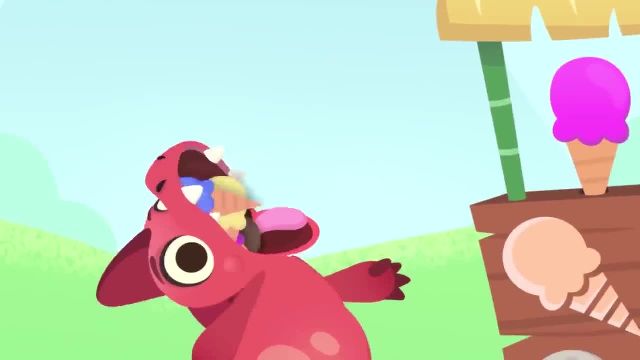 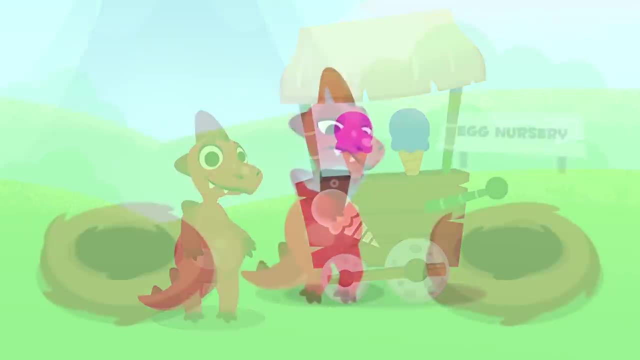 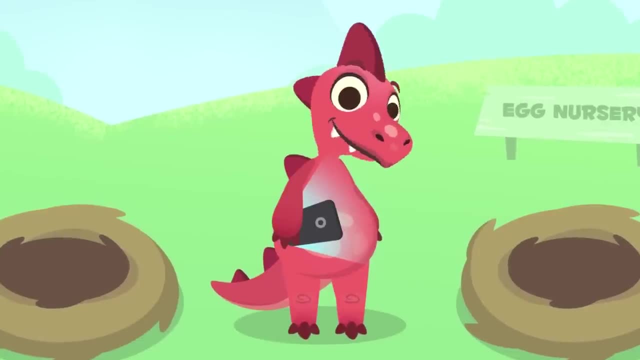 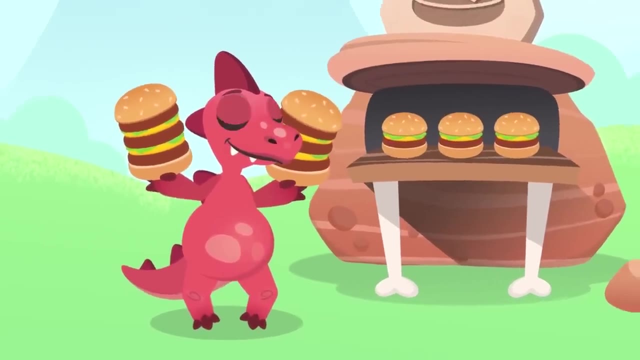 I'm not. Are you bored? Shall we go get some delicious dinner. Look at those super hamburgers you got yourself, Dino, It'll take you a while to eat them. Wow, you really were hungry. Now that we're full, we can practice some additions. 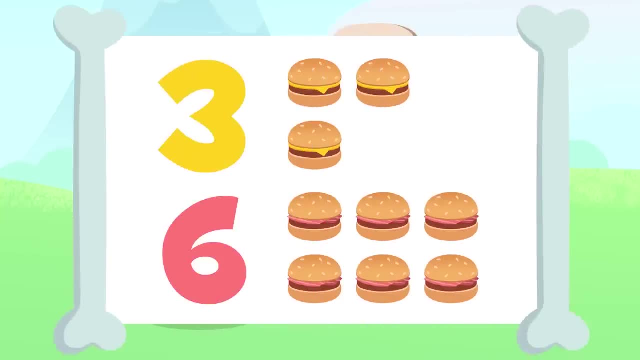 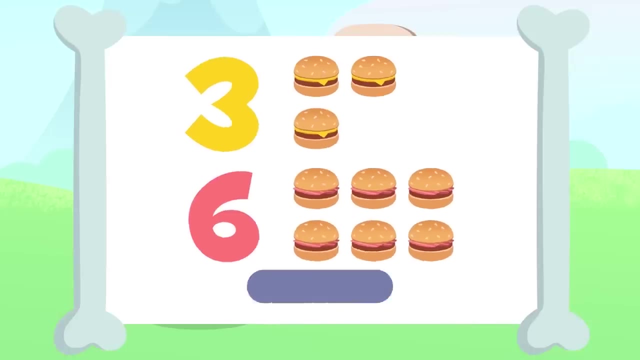 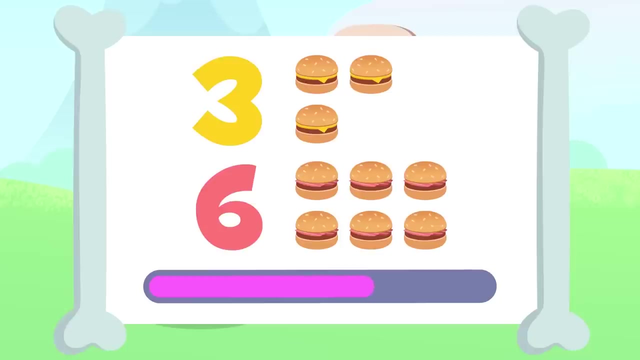 What do you think? Come on, let's add. How many hamburgers are there? Up here we have three and down there six. Go ahead, You do the adding. I'll give you a few seconds. You got it. 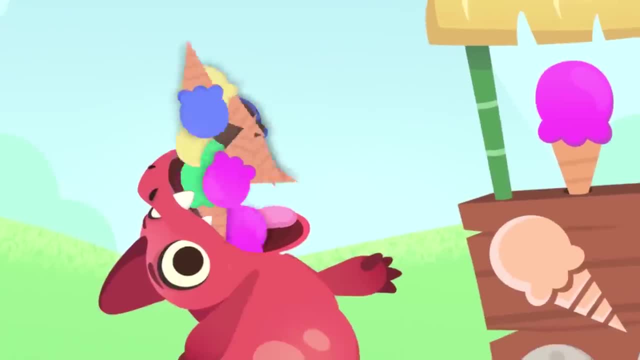 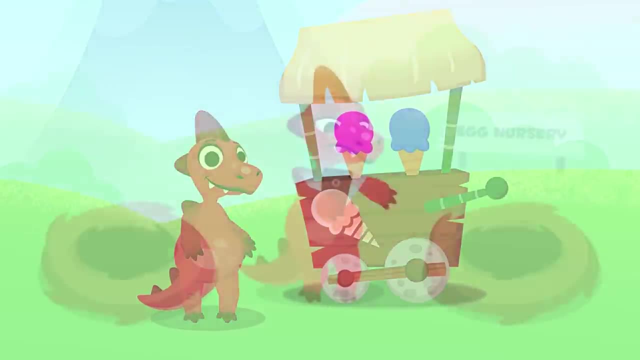 You're going to feel sick, Dino. Wouldn't it be best if you save it for later? My, my Dino, You're never full. Hey, Dino, How's it going? I see you're not doing much today either. Are you bored? Shall we go get. 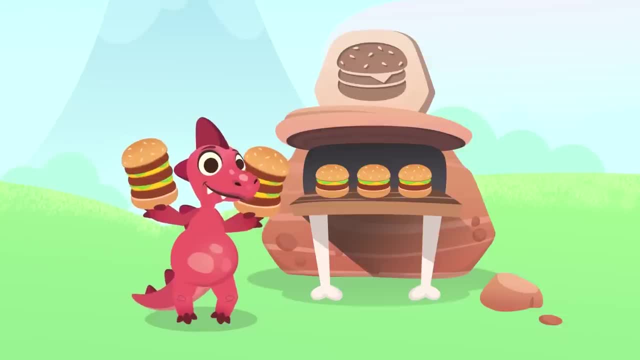 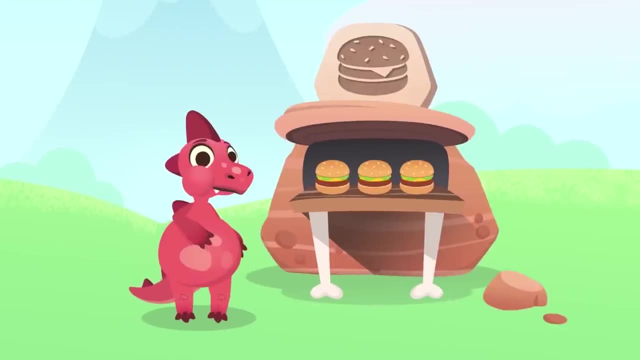 some delicious dinner. Look at those super hamburgers you got yourself, Dino, It'll take you a while to eat them. Wow, you really were hungry. Now that we're full, we can practice some additions. What do you think? Come on, let's add. How many hamburgers are there? 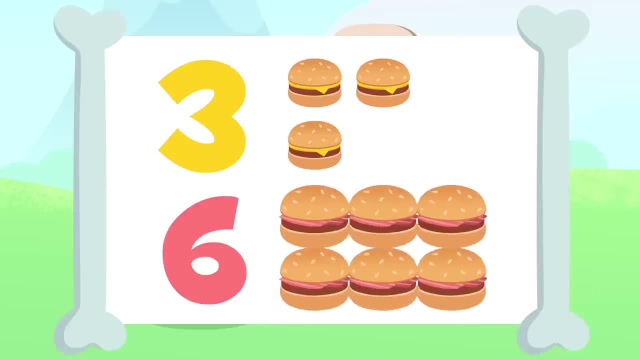 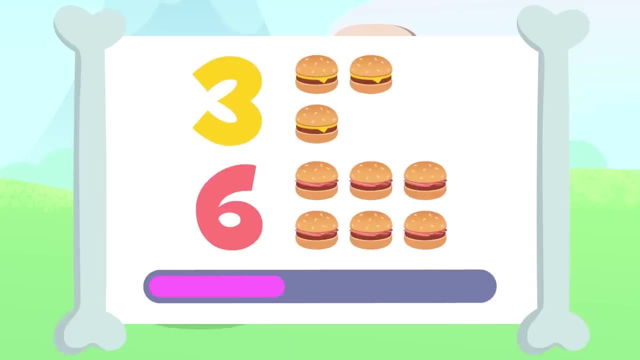 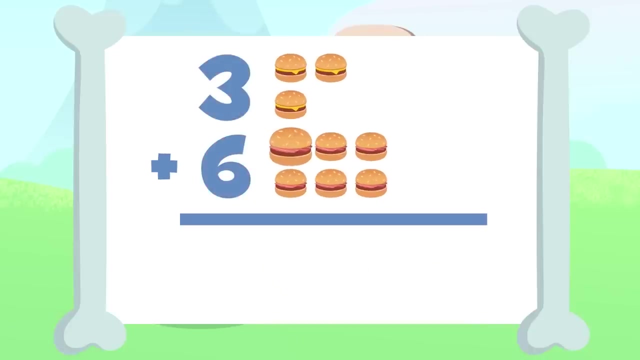 Up here we have 3, and down there 6.. Go ahead, you do the adding. I'll give you a few seconds. You got it. Let me try. All hamburgers together would be 1,, 2,, 3,, 4,, 5,, 6,, 7,, 8, and 9.. 9! We have 9 hamburgers. 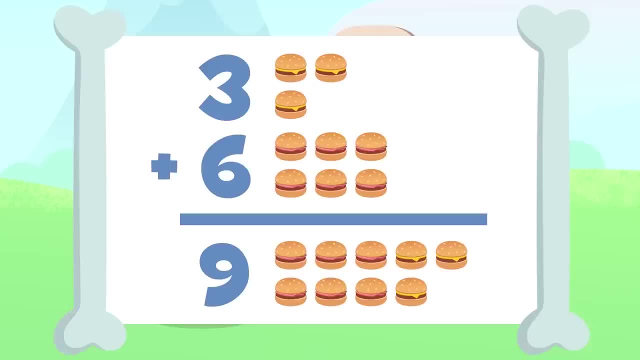 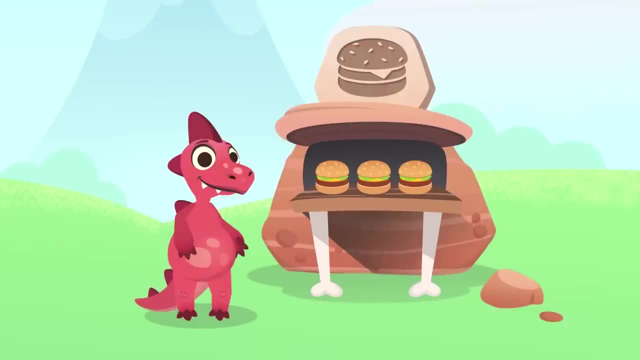 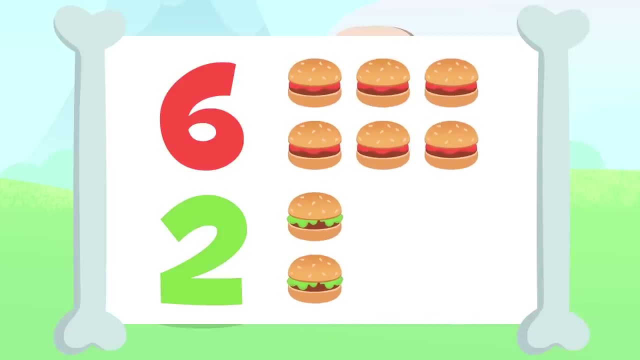 3 plus 6 equals 9.. Our first addition: The result of adding 3 plus 6 is equal to 9.. Well done, Dino. Let's try another one. There are 6 hamburgers up here and 2 down there. Why don't you add them up? Take your time. 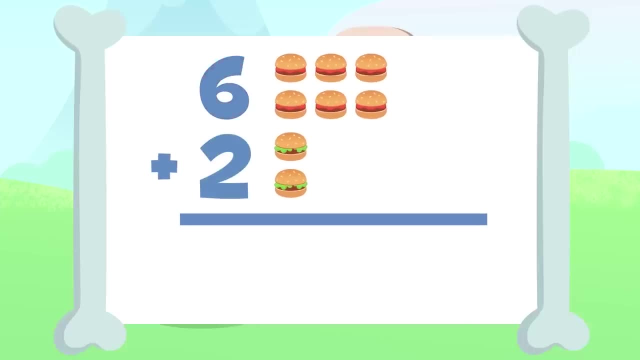 You got it. If we add up these hamburgers, we'll have 1,, 2,, 3,, 4,, 5,, 6,, 7, and 8.. 8! We have 8 hamburgers in total, 6 plus 2 equals. 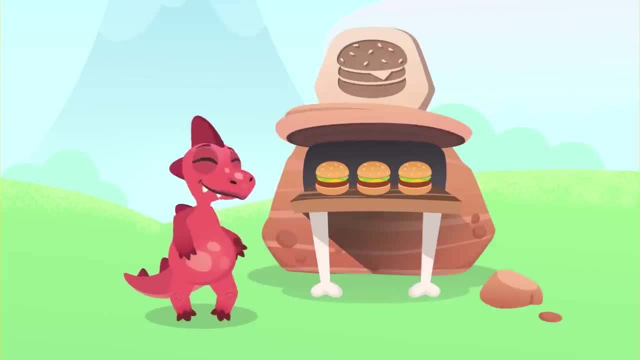 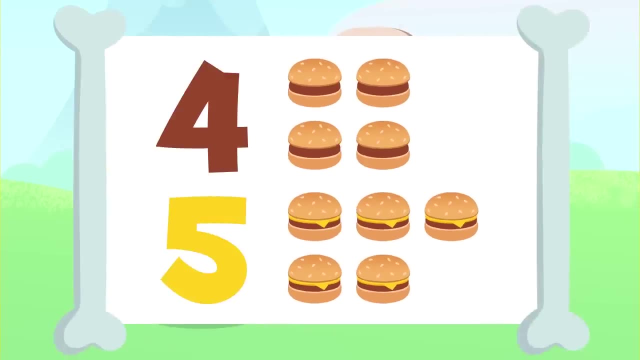 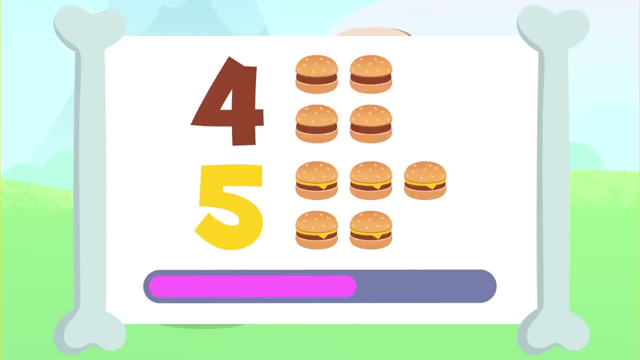 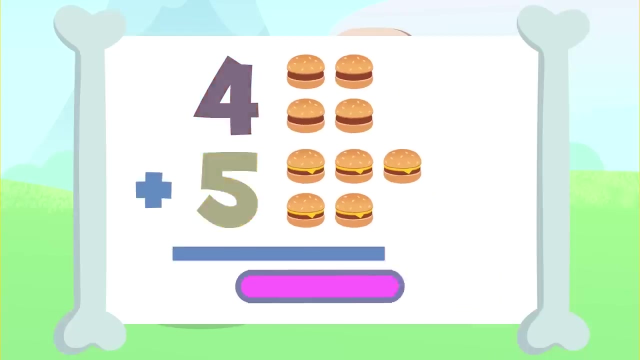 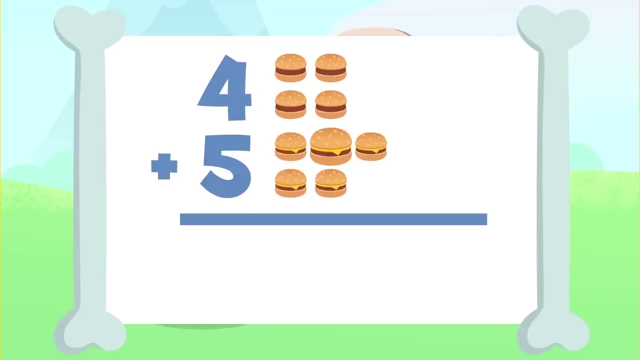 8.. Shall, we carry on. Now you'll have to add these 4 hamburgers up here to those 5 hamburgers down there. I'll give you a few seconds to add them up. How did it go? You have it. The results of adding 4 plus 5 is 1, 2,, 3,, 4,, 5,, 6,, 7,, 8, and. 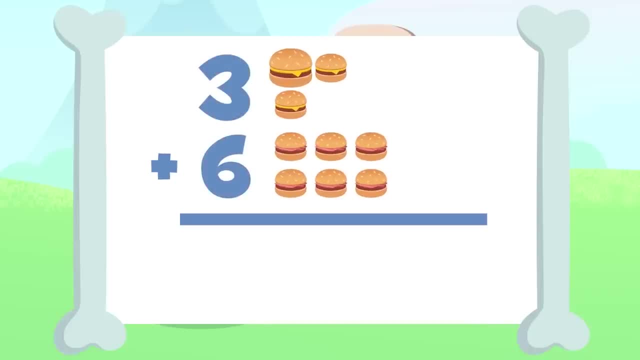 Let me try. All hamburgers together would be 1,, 2,, 3,, 4,, 5,, 6,, 7,, 8, and 9.. 9! We have 9 hamburgers. 3 plus 6 equals 9.. 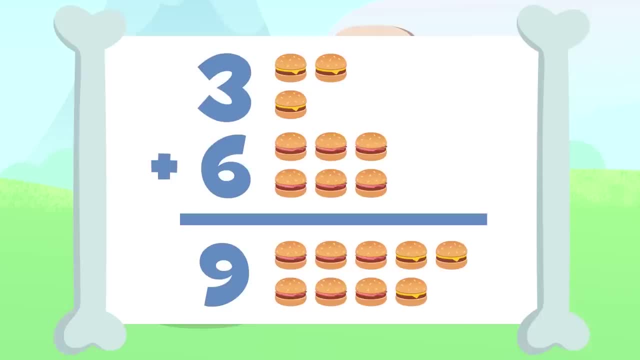 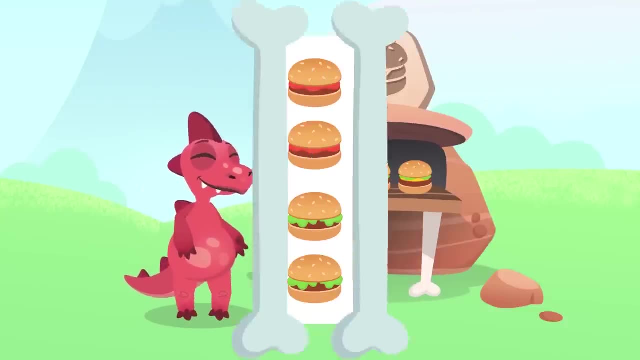 We just did our first addition. The result of adding 3 plus 6 is equal to 9.. Well done, Dino. Let's try another one. There are 6 hamburgers up here and 2 down there. Why don't you add them up? 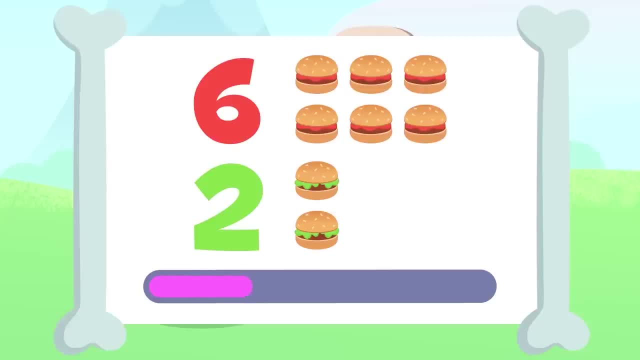 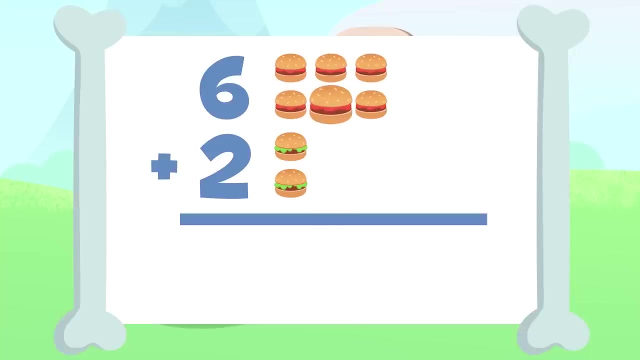 Take your time, You got it. If we add up these hamburgers, we'll have 1,, 2,, 3,, 4,, 5,, 6,, 7, and 8.. 8!- We have 8 hamburgers in total. 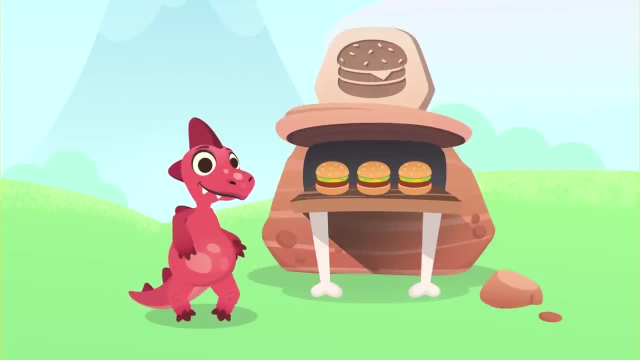 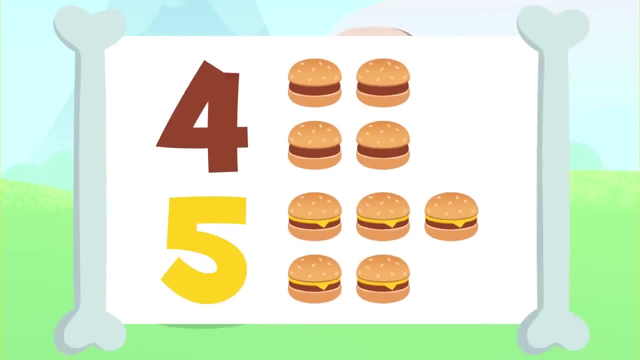 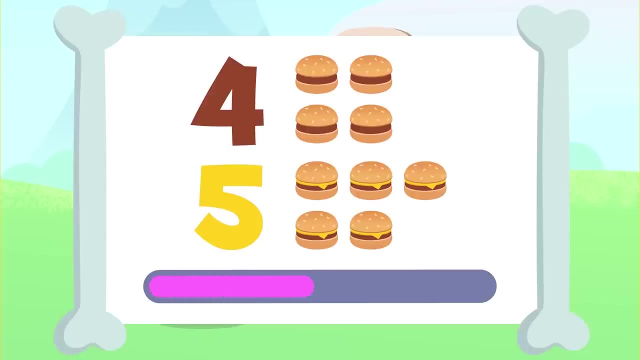 6 plus 2 equals 8.. Shall, we carry on. Now you'll have to add these 4 hamburgers up here to those 5 hamburgers down there. I'll give you a few seconds to add them up. How did it go? 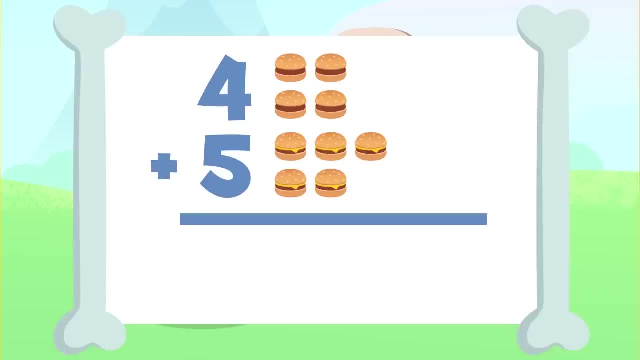 You have it. The result of adding 4 plus 5 is 1,, 2,, 3,, 4,, 5,, 6,, 7,, 8, and 9.. 9! We have 9 hamburgers. 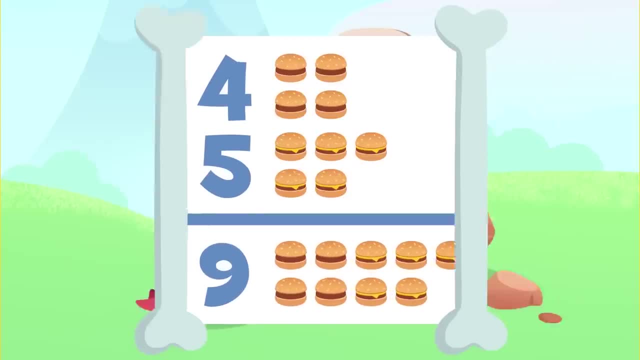 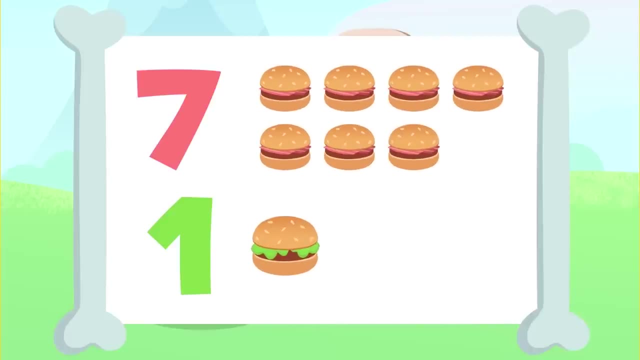 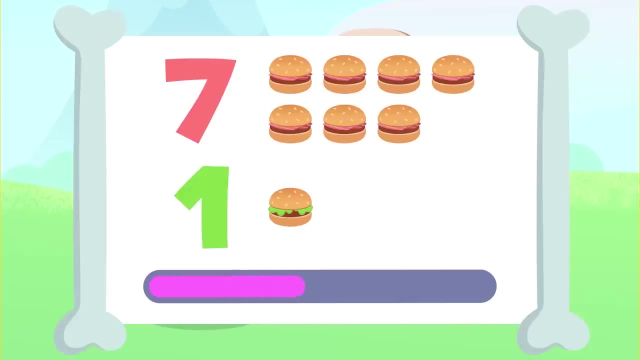 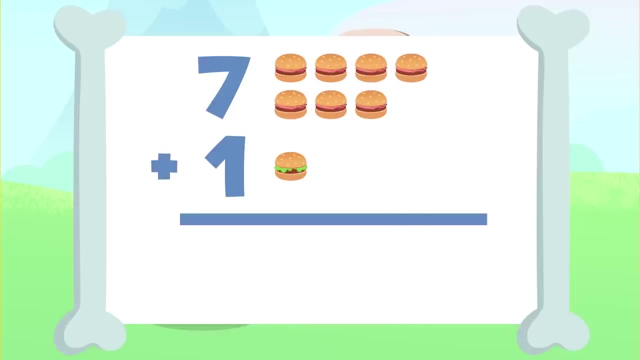 4 plus 5 is equal to 9.. Let's try another one. You'll have to add these 7 hamburgers up here to that 1 hamburger down there. Let's go for it. You got it. The result of adding 7 plus 1 is 1,, 2,, 3,, 4,, 5,, 6, 7, and 8.. 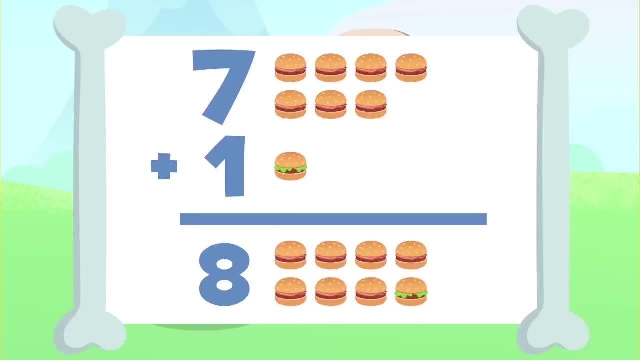 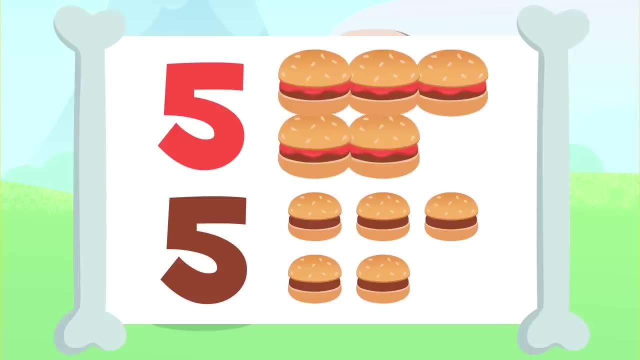 8!. There are 8 hamburgers. 7 plus 1 is equal to 8.. Shall, we do the last one. We have to add these 5 hamburgers up here to the 5 hamburgers down there. Let's go for it. 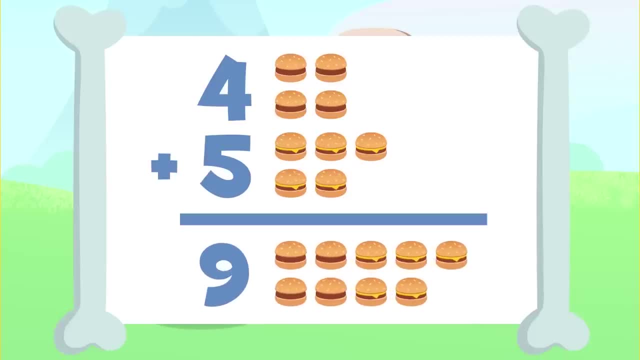 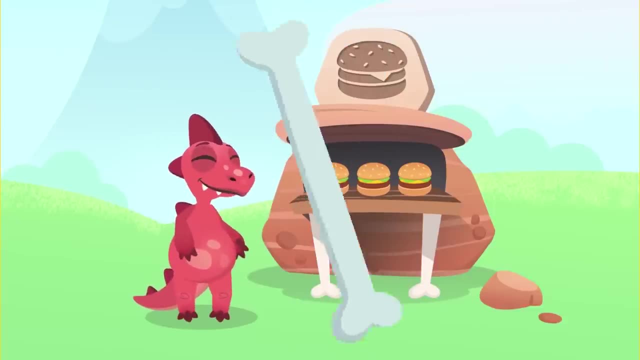 9. 9! We have 9 hamburgers. 4 plus 5 is equal to 9.. Let's try another one. You'll have to add these hamburgers up here to that one hamburger down there. Let's go for it. 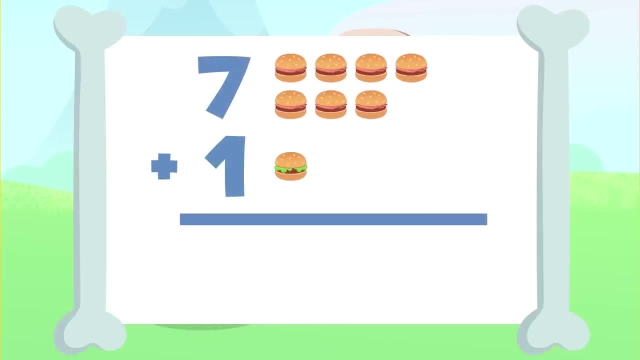 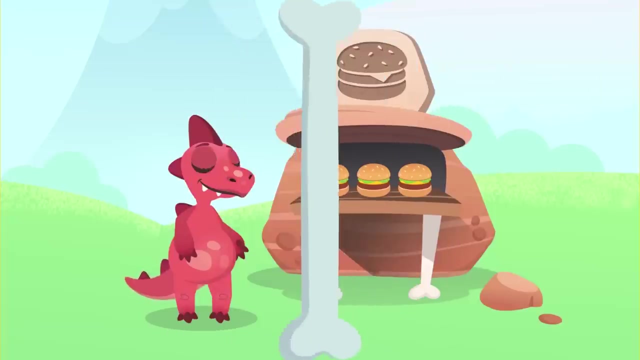 You got it. The result of adding 7 plus 1 is 1,, 2,, 3,, 4,, 5,, 6,, 7, and 8.. 8!, There are 8 hamburgers. 7 plus 1 is equal to 8.. Shall, we do the last one. We have to add these 5. 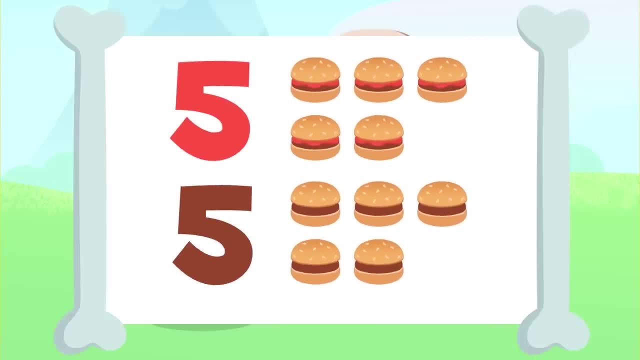 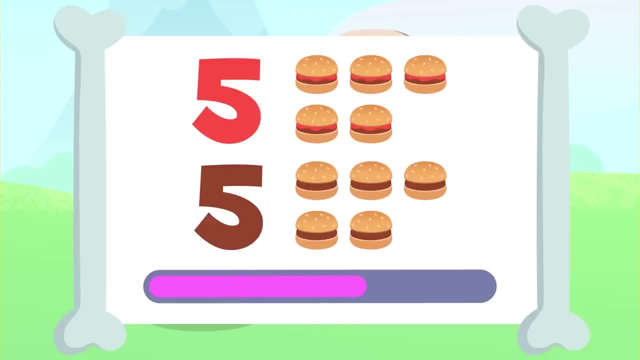 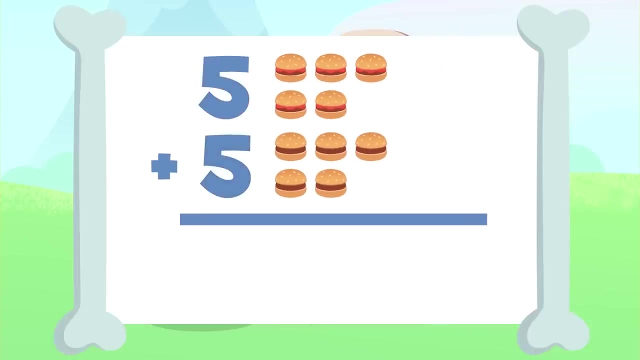 hamburgers up here to the 5 hamburgers down there. Let's go for it. That's it. The result of adding 5 plus 5 is 1, 2, 3, 4, 5, 6, 7,, 8, 9, and 10.. 10! There are 10 hamburgers. 5 plus 5 equals 10.. 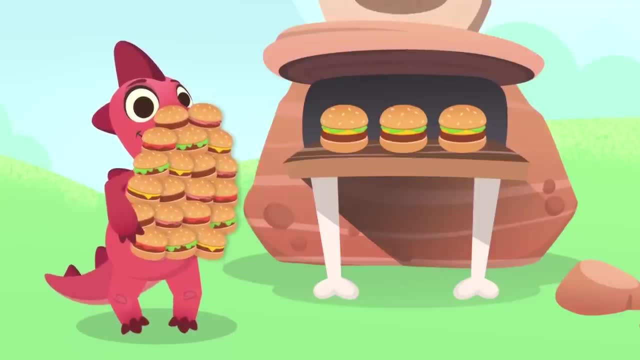 Dino, what are you going to do with all those hamburgers? Are you going to eat them? You're going to feel sick, Dino. Wouldn't it be best if you save them for later? My, my Dino. 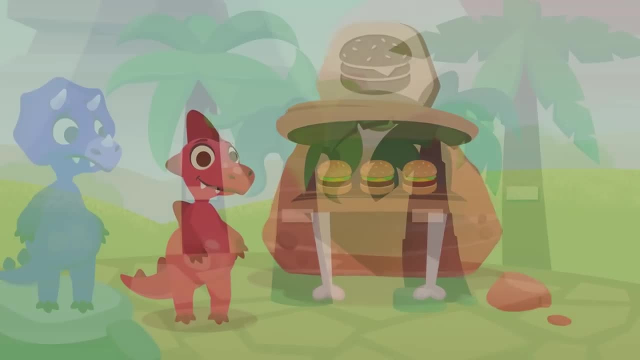 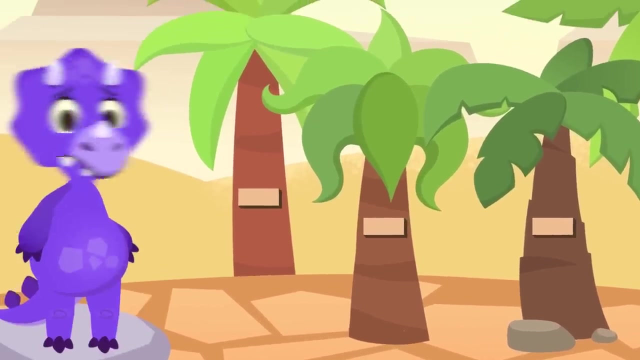 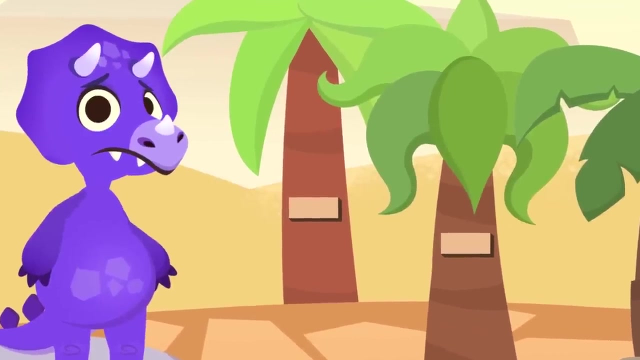 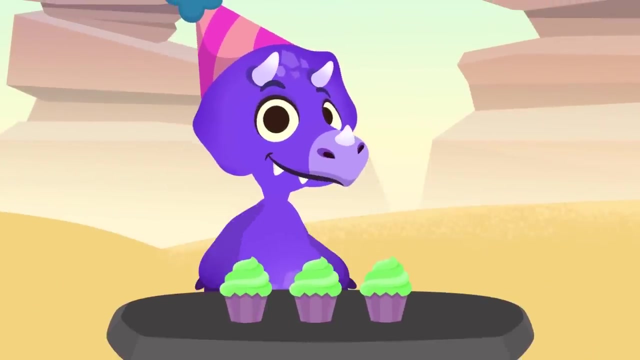 you're never full. Hey, sorry, What's the matter? I see you're worried. Do you know what all those lines are for? You don't. They're the subtraction symbol, the minus sign. Do you know how to subtract? Don't worry, sorry, I'll teach you how. Whoa These. 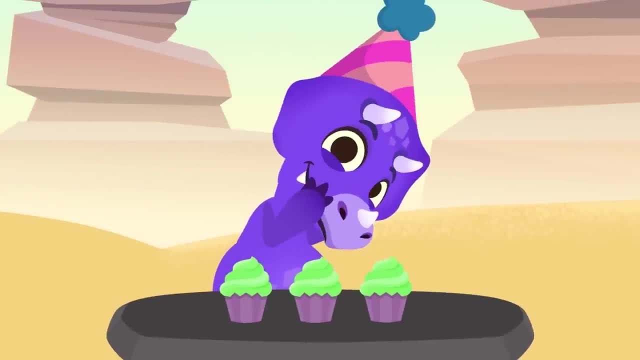 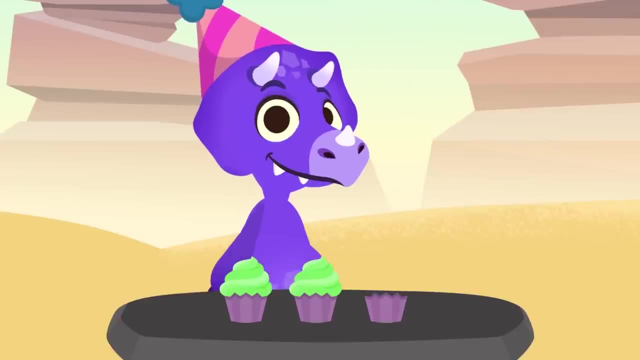 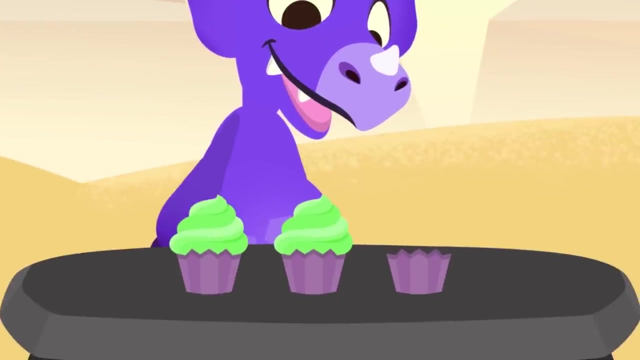 cupcakes look awesome. sorry, What is it? Are you hungry? Come on, don't be shy, Have one In one bite. You're never full. sorry, Do you know? you've just done a subtraction without realizing it. We subtract to know. 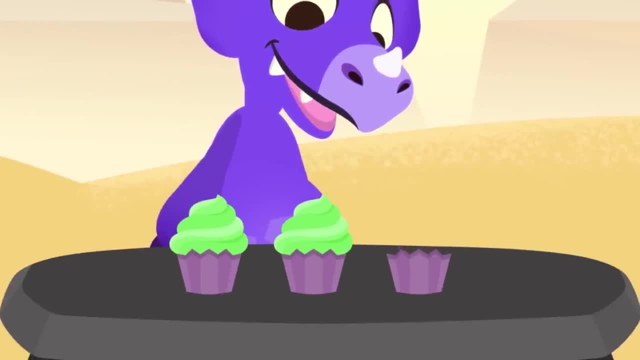 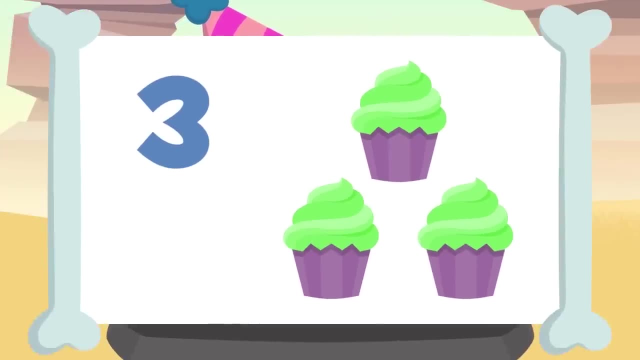 how many things we have left after taking away some of them, just like you did with these cupcakes. For example, before there were three cupcakes on the table and you've eaten one. So if we take one away from three, there will be one and two cupcakes left. Three. 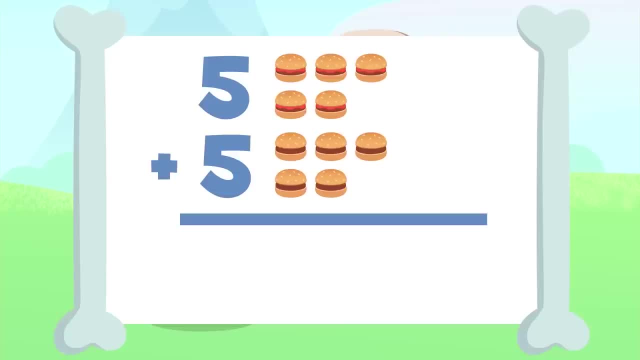 That's it. The result of adding 5 plus 5 is 1,, 2,, 3,, 4,, 5,, 6,, 7,, 8,, 9, and 10.. 10!: There are 10 hamburgers. 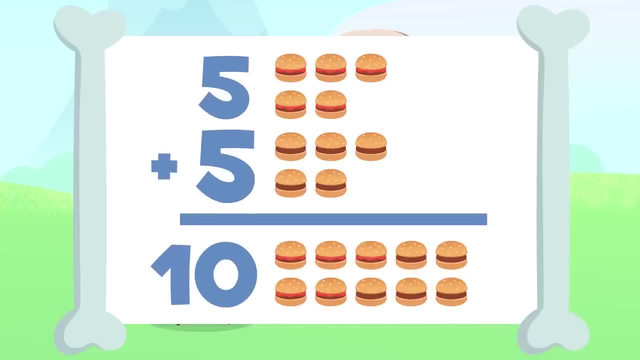 5 plus 5 is equal to 10.. Dino, what are you going to do with all those hamburgers? Are you going to eat them? You're going to feel sick, Dino. Wouldn't it be best if you save them for later? 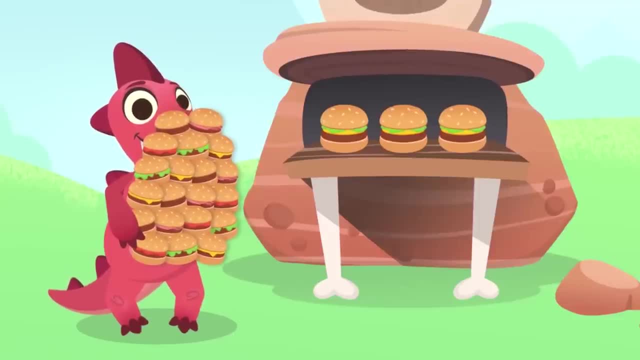 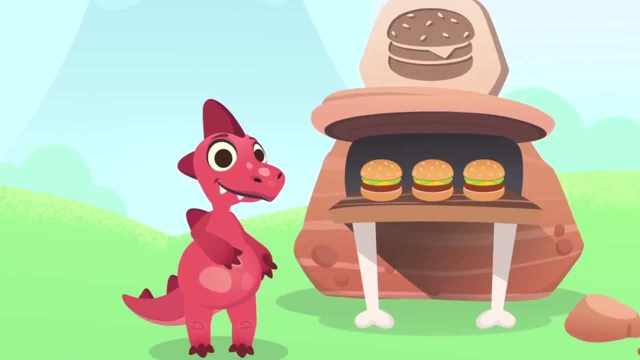 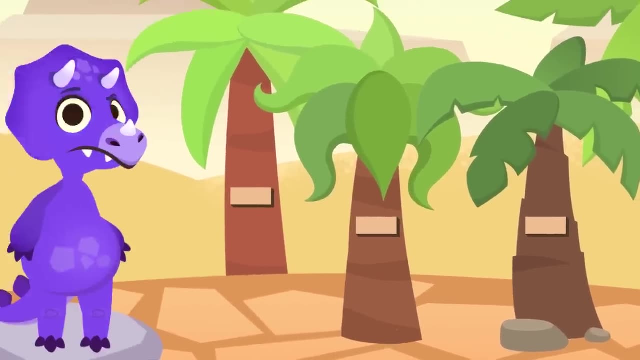 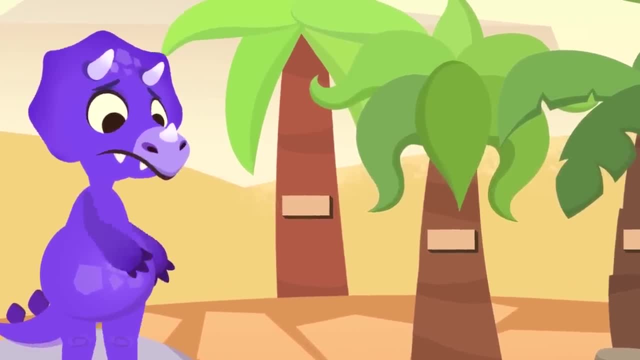 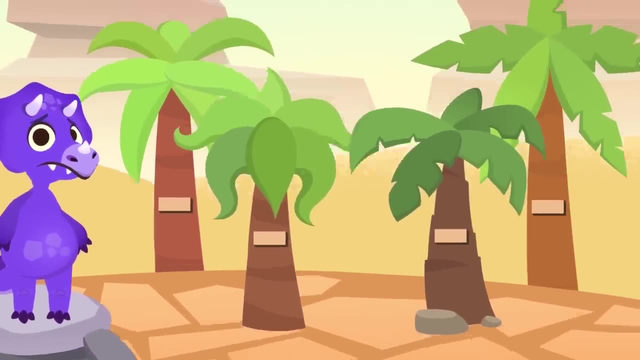 You don't. They're the subtraction symbol, The minus sign. Do you know how to subtract? Uh-uh, Uh-uh, Don't worry, Sorry, I'll teach you how. Whoa, These cupcakes look awesome, Sorry. 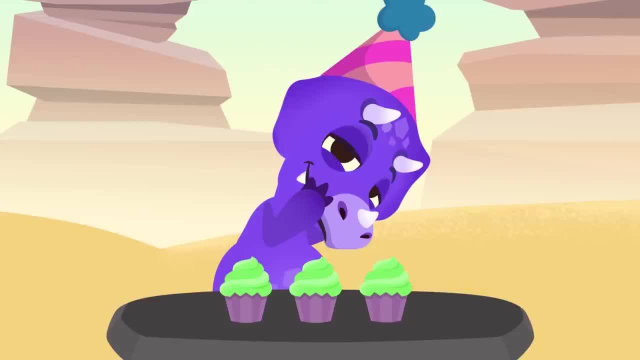 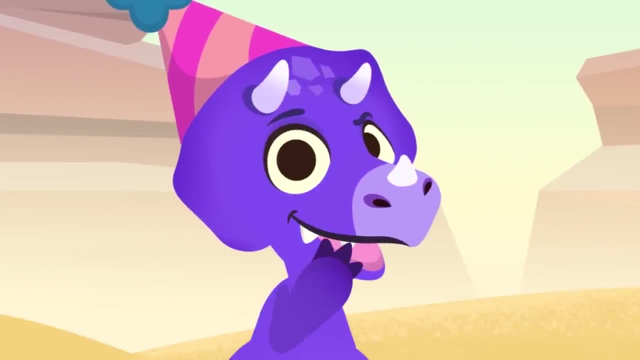 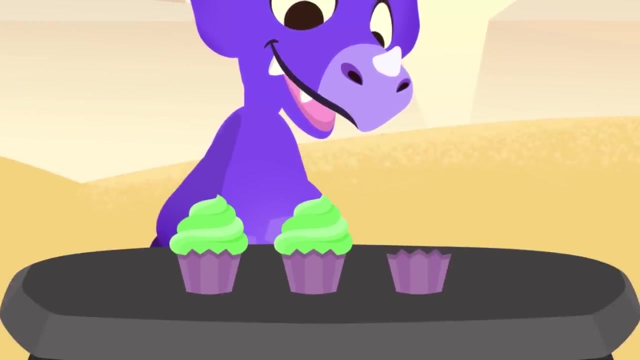 What is it? Are you hungry? Come on, don't be shy, Have one In one bite. You're never full. Sorry, Do you know? you've just done a subtraction without realizing it. We subtract to know how many things we have left after taking away some of them just. 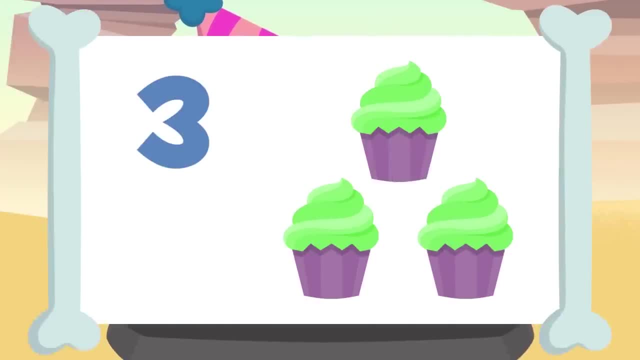 like you did with these cupcakes. For example, before there were three cupcakes on the table and you've eaten one. So if we take one away from three, there will be one and two cupcakes left. Three minus one equals two. Well done. 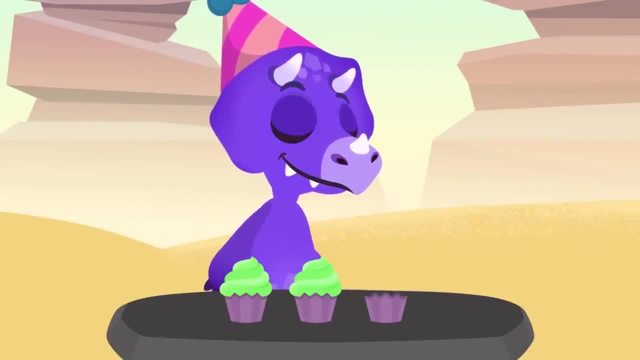 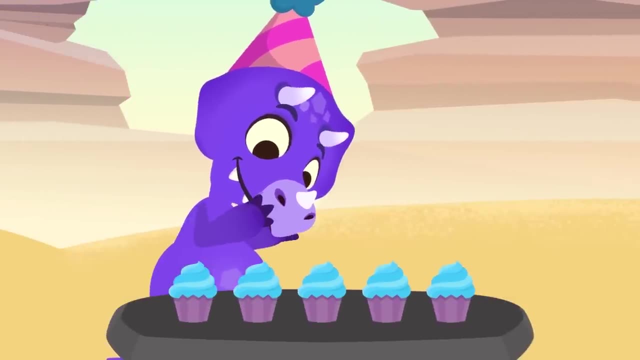 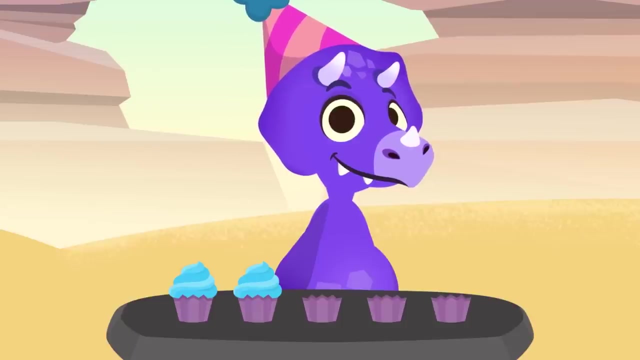 We have done our first subtraction. See how easy it was. Yum, yum, These cupcakes are mouthwatering. But wait, Sorry, You've subtracted again without realizing How many are there left. this time There were five cupcakes and you've eaten three. 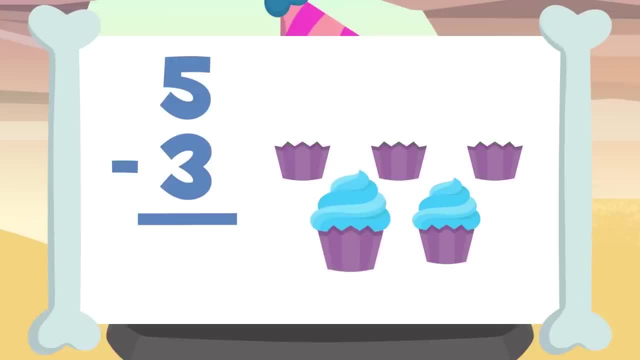 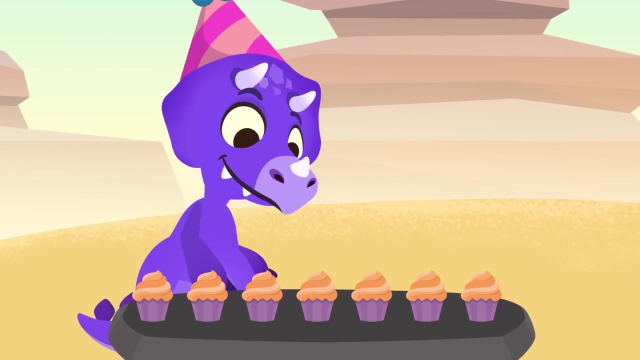 So if we take away three from five, there will be one and two cupcakes left. Two. Five minus three equals two. Well done, two Awesome. Are you still hungry? There's nothing we can do with you, sorry, is there? 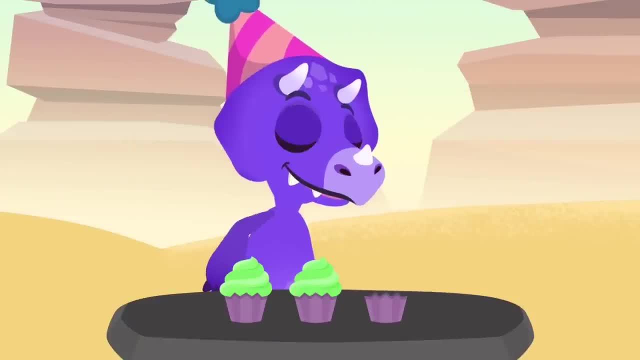 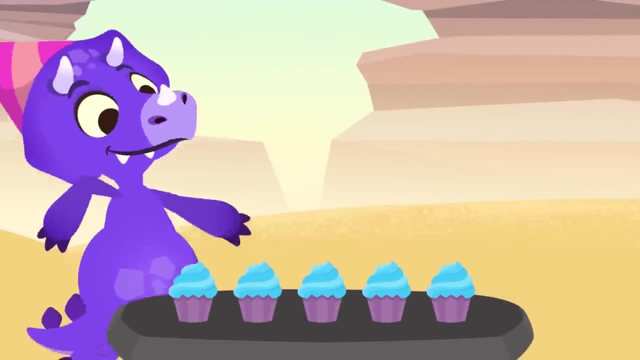 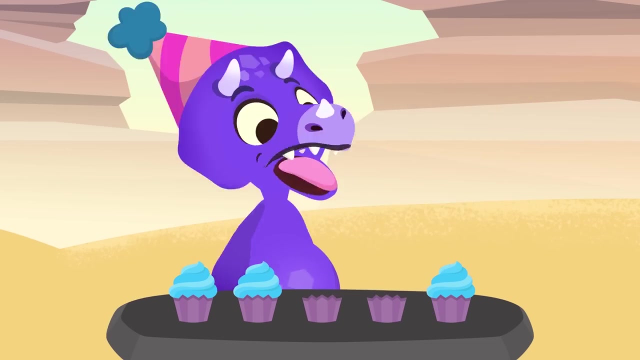 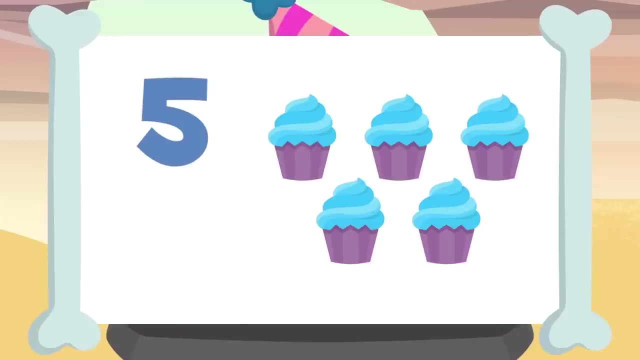 minus one equals two. Well done, No subtraction. See how easy it was. Yum yum. These cupcakes are mouth-watering. But wait, Sorry, You've subtracted again without realizing How many are there left. this time There were five cupcakes and you've eaten three. 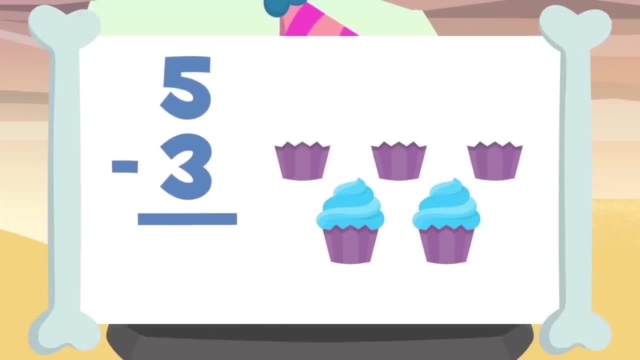 So if we take away three from five, there will be one and two cupcakes left. Two, five and three. You're truly psychotic, sorry. Two Two, Two, Two, Five minus three equals two. Awesome, Are you still hungry? 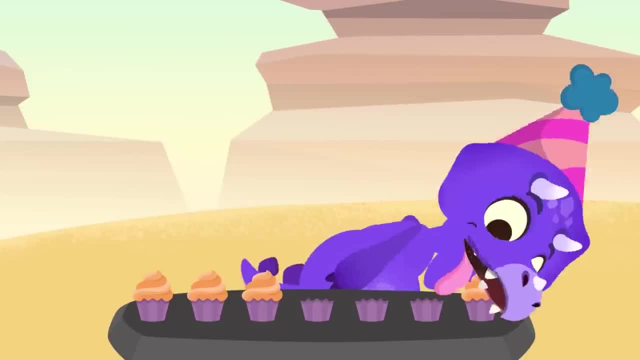 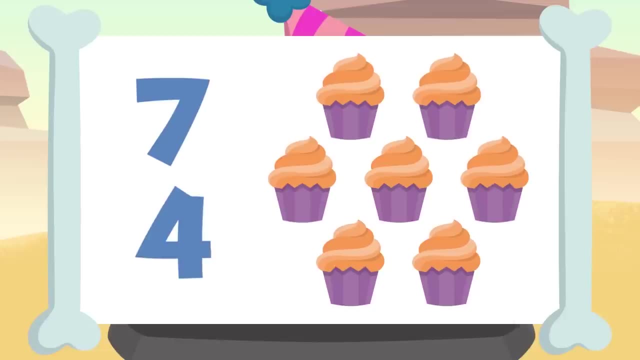 There's nothing we can do with you. sorry is there On the table there were seven cupcakes and you've eaten four of them. If we take away four from seven, one, two, three and four, the result is one, two and three. 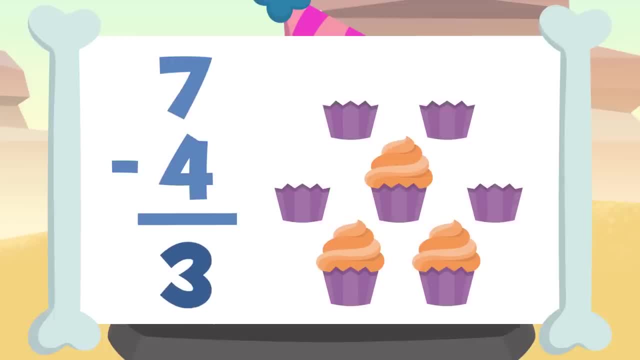 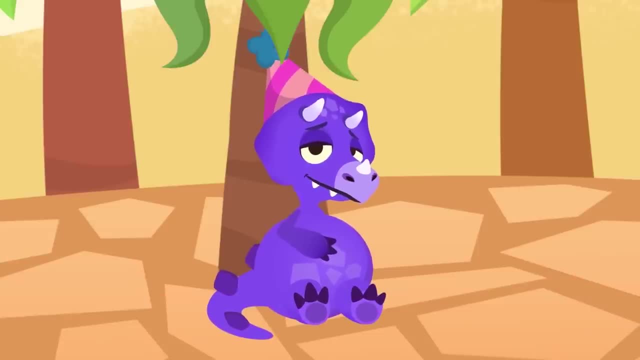 Three Seven minus four equals three. Good job, sorry. Do you like subtracting? I told you sorry, there were too many cupcakes. Well, let's recap the subtractions we practiced today. alright, We can also do horizontal subtractions. 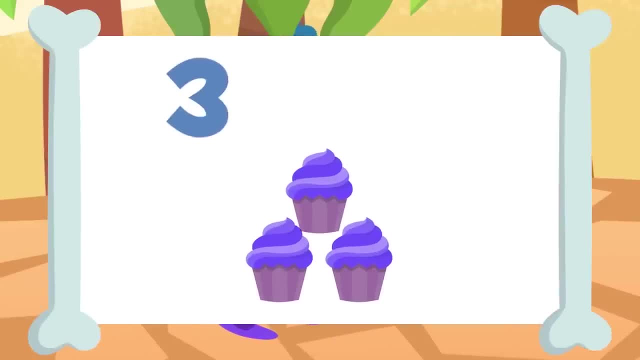 It's done in the same way. Pay attention: Three minus one equals one and two. Three minus one equals two. Awesome, Let's do the next one. If I take away the three cupcakes from these five cupcakes- one, two and three- I will be left with one and two cupcakes. 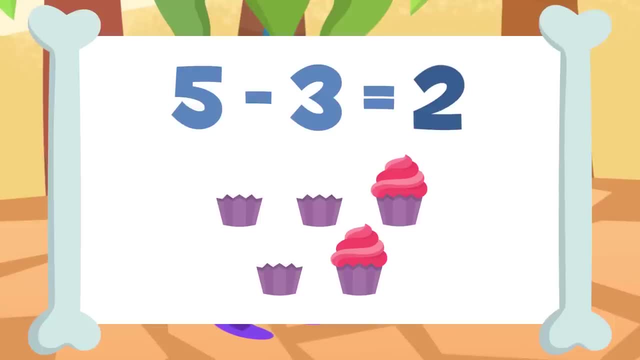 Five minus three equals equals two. Excellent, sorry Shall we try the last one. If I take away the four cupcakes from these seven cupcakes- one, two, three and four- I will be left with one, two and three. 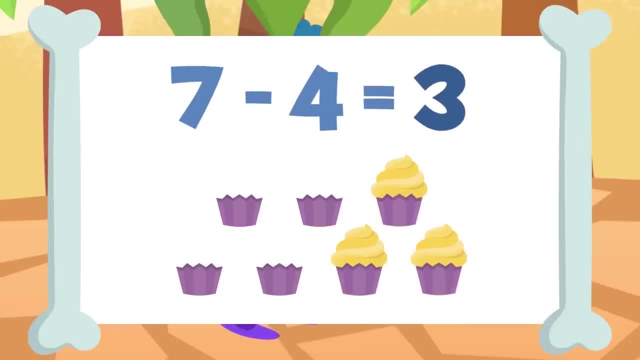 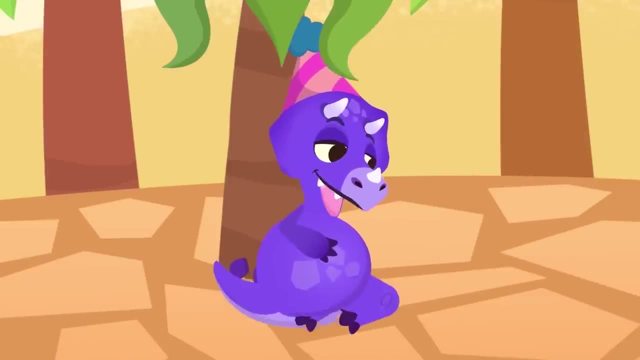 Seven minus four equals three. Well done, sorry. Now you know how to subtract. Are you feeling better? sorry, Uh-uh, Uh-uh, Uh-uh, Uh-uh, Uh-uh, Uh-uh, Uh-uh. 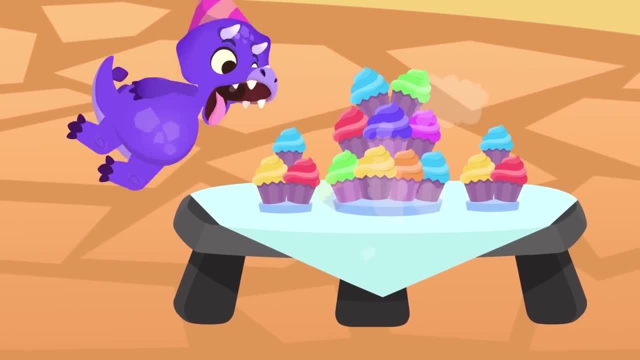 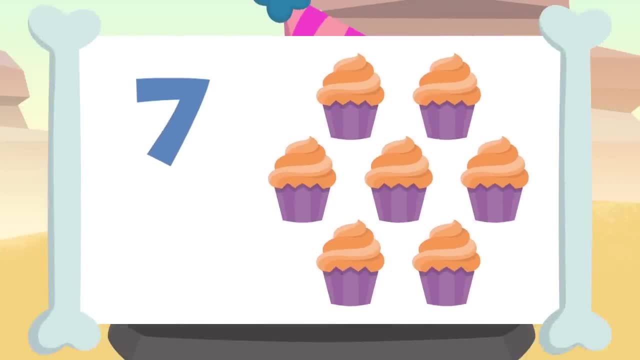 On the table. there were seven cupcakes and you've eaten four of them. If we take away four from seven, one, two, three and four, the result is one, two and three, Three, Seven minus four equals three. Good job, sorry, Do you like subtracting? 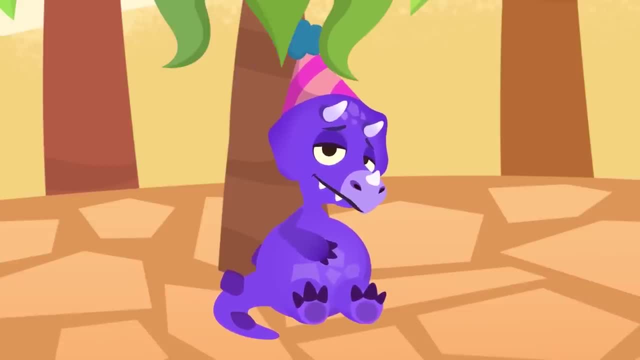 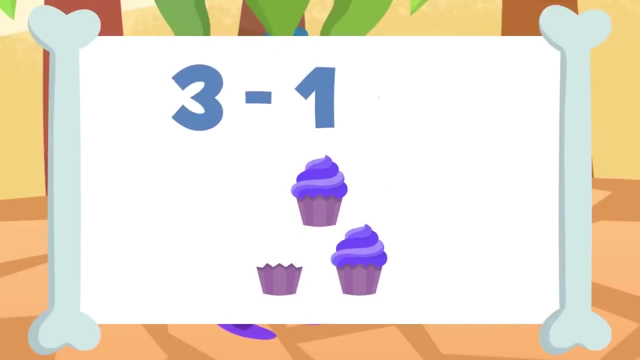 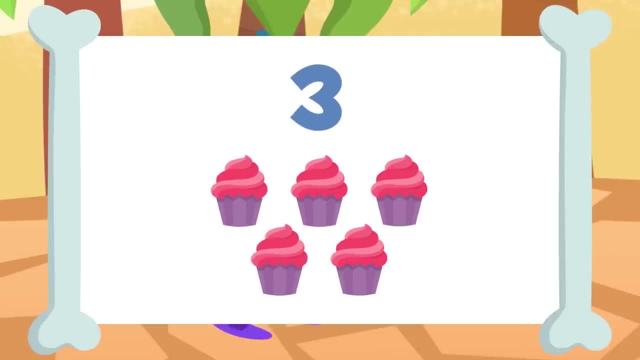 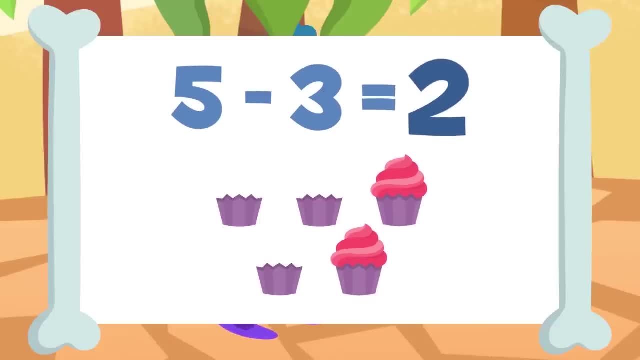 cupcakes. five minus three equals two. excellent, sorry, shall we try the last one. if i take away the four cupcakes from these seven cupcakes- one, two, three and four- i will be left with one, two and three. seven minus four equals three. well done, sorry. now you know how to subtract. 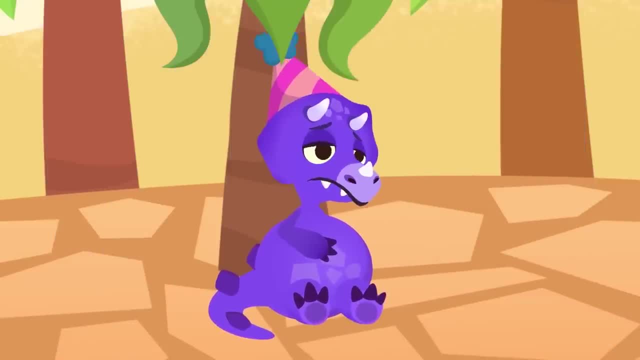 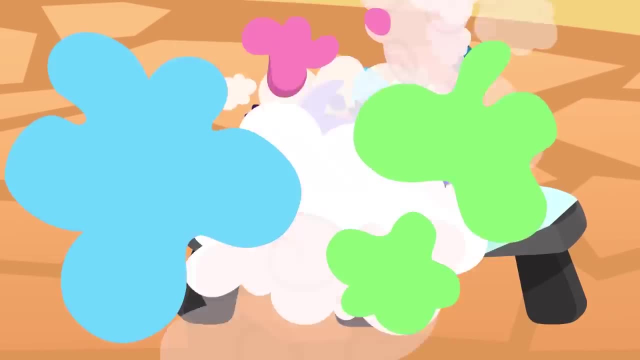 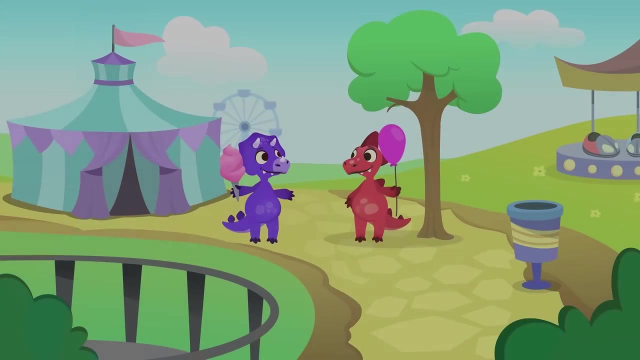 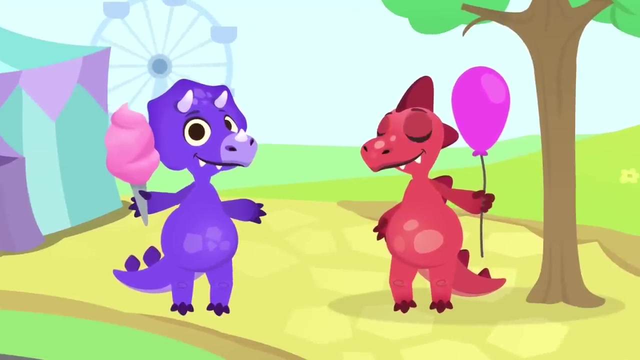 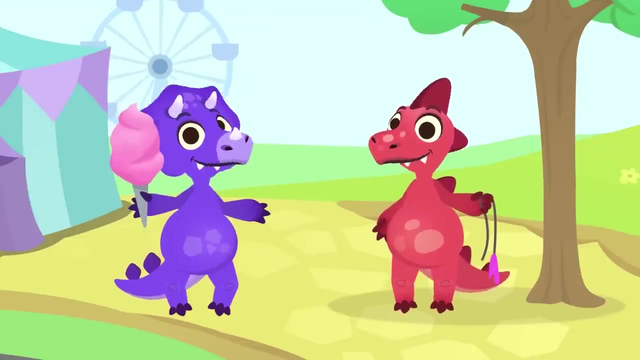 are you feeling better? sorry, sorry, hi everyone. this theme park is just. this theme park is just Just awesome. Are you having a good time? Oopsie, Your balloon just bursted. Shall we go get you another one. What are you playing? You've got perfect aim. 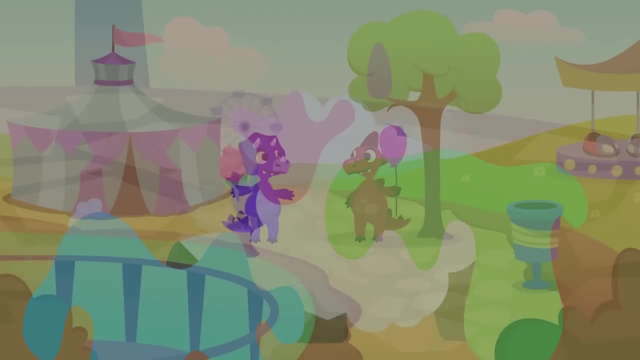 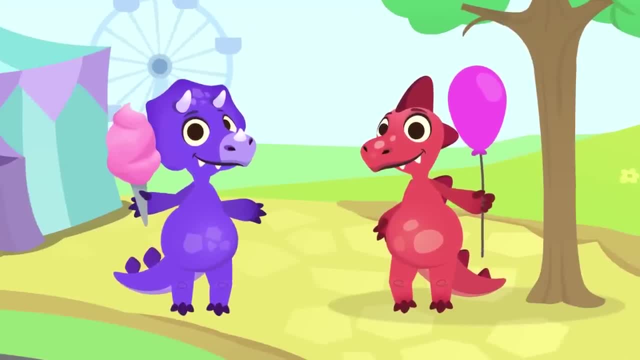 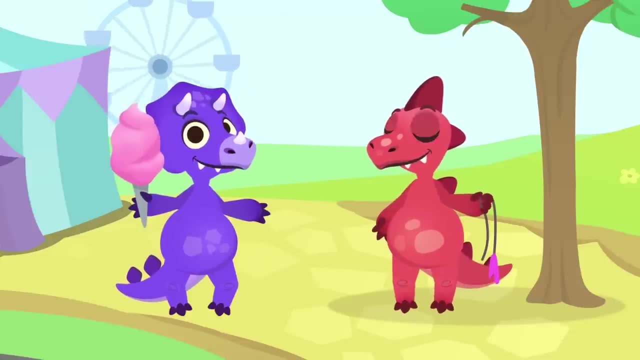 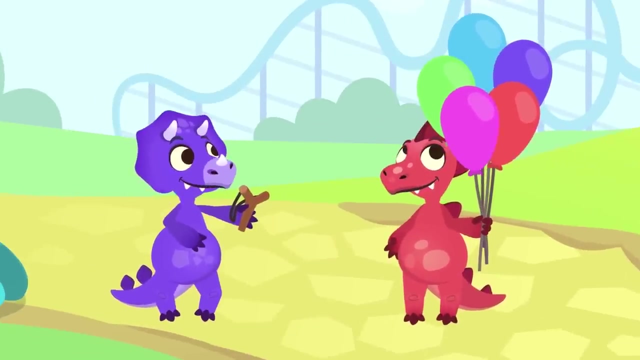 This theme park is just awesome. Are you having a good time? Oopsie, Your balloon just busted. Uh-uh, Uh-uh, Shall we go get you another one. What are you playing? Uh-uh, You've got perfect aim. 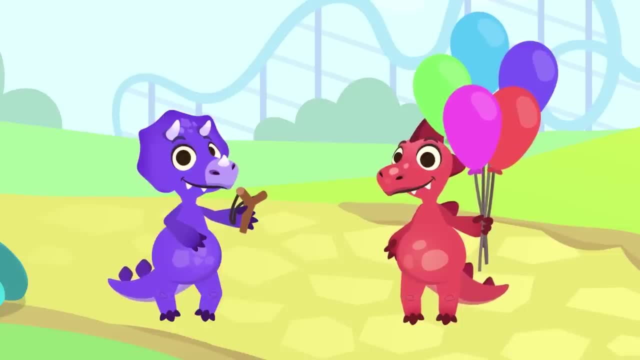 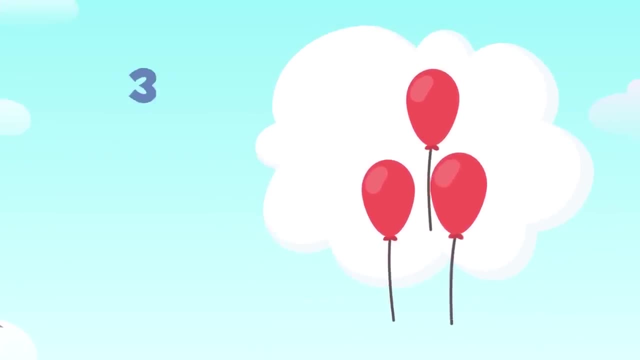 That's a great way to learn how to do subtractions. Would you like to practice for a while? Let's find out how good my aim is. There are one, two and three balloons and I'm going to see if I can burst one of them. 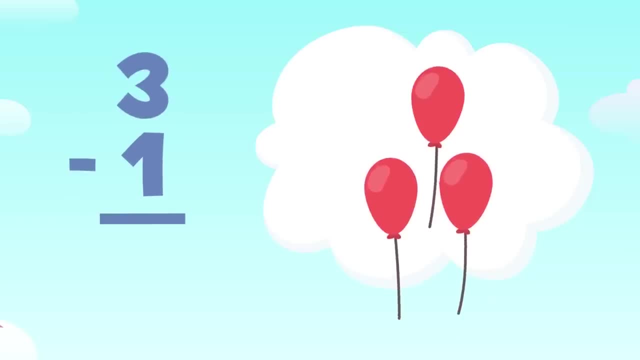 The subtraction we need to do is three minus one. This means there are three balloons and I have to burst one. I'm going to aim well to see how many I'll have left. Fantastic, I aimed well, Let's see how many there are now. 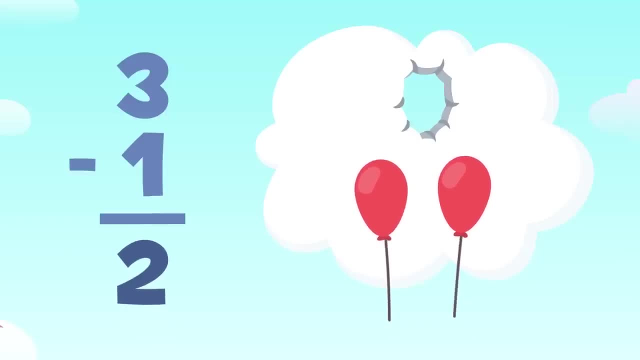 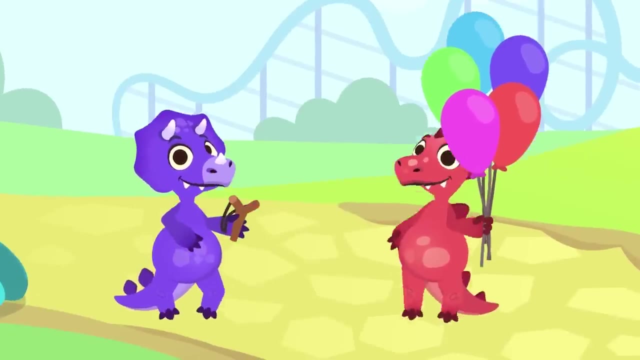 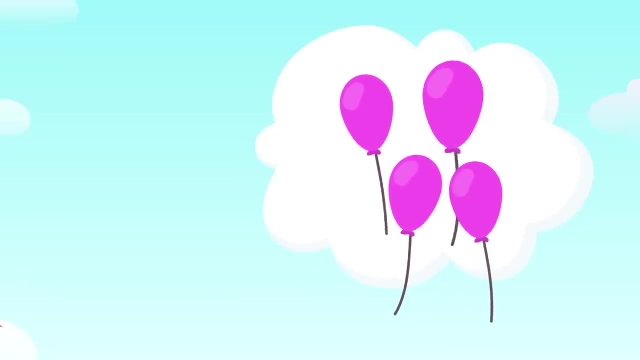 One and two. There are two balloons left. The result of subtracting three from one equals two. My aim is truly good. Hahaha, Some balloons are flying away. There are one, two, three and four balloons and I'm going to try to aim at two of them. 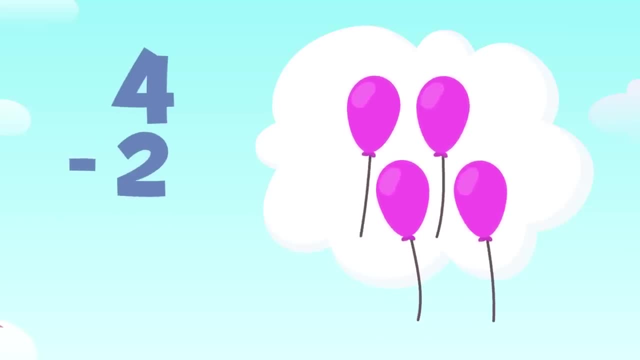 How many balloons will there be left? We need to subtract four minus two. This means that out of four balloons we need to take away two. I'm going to aim well to see how many I'll have left. One and two. One and two. 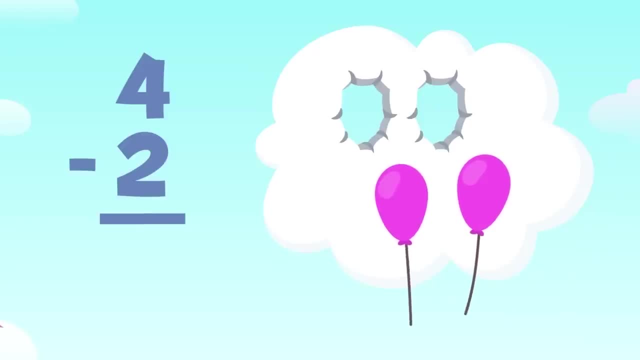 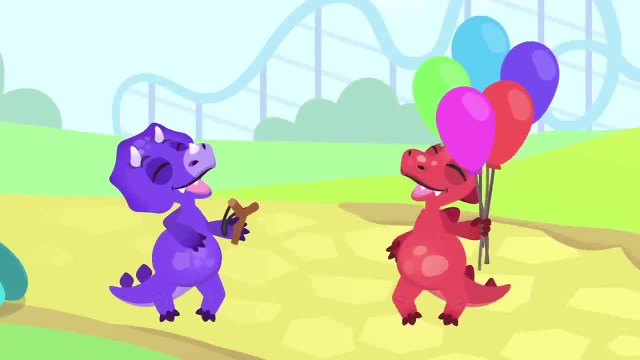 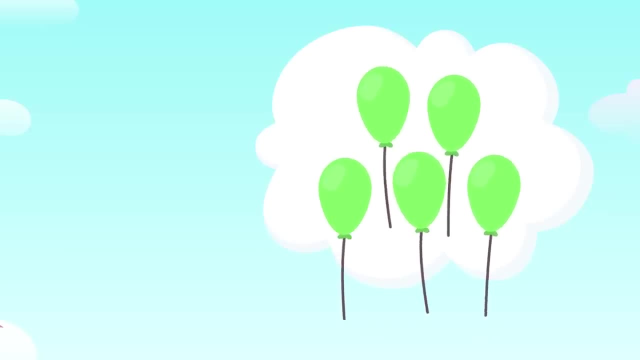 I'm so good at shooting the slingshot. Hahaha, You've let more balloons fly away. There are one, two, three, four and five balloons. How many balloons are left? One and two. One and two. One and two. 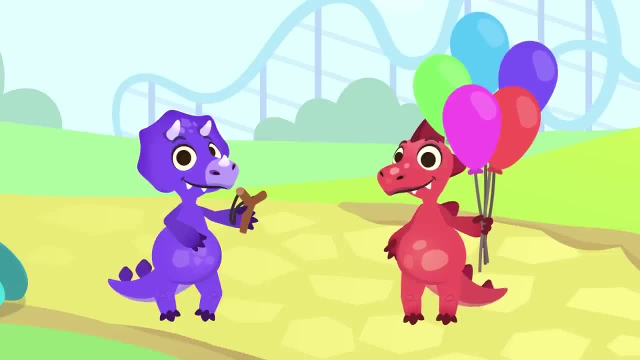 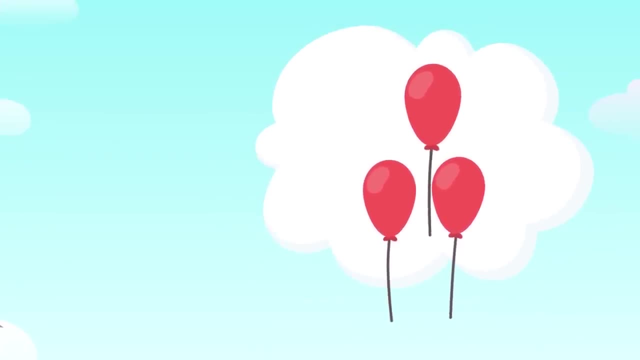 That's a great way to learn how to do subtractions. Would you like to practice for a while? Let's find out how good my aim is. There are one, two and three balloons And I'm going to see if I can burst one of them. 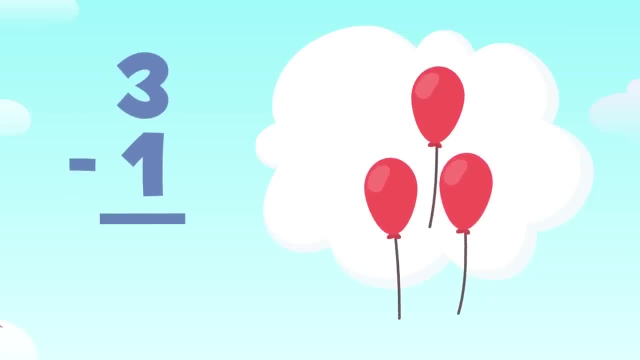 The subtraction we need to do is three minus one. This means there are three balloons and I have to burst one. I'm going to aim well to see how many I'll have left. Fantastic, I aimed well, Let's see how many there are now. 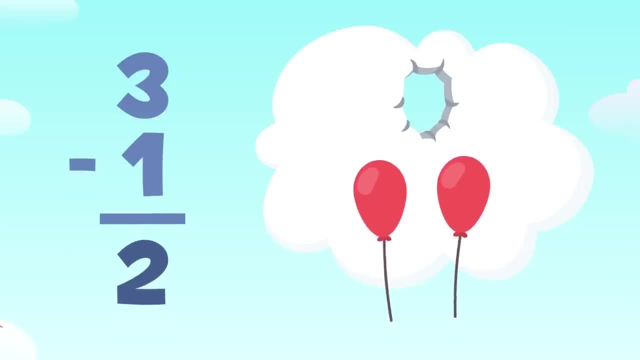 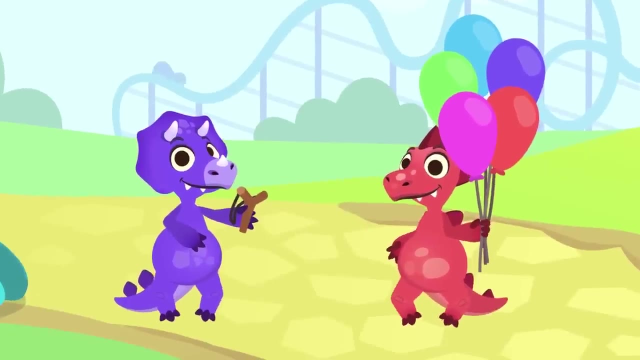 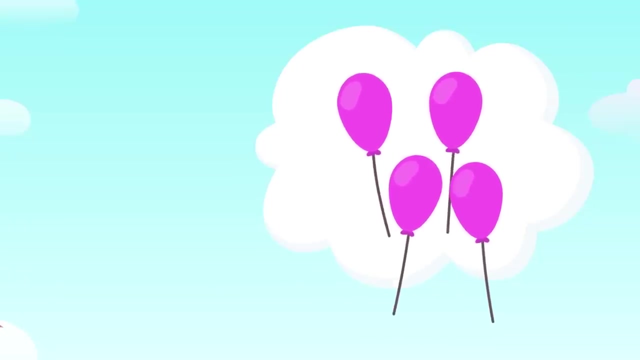 One And two. There are two balloons left. The result of subtracting three from one equals two. My aim is truly good. Some balloons are flying away. There are one, two, three and four balloons And I'm going to try to aim at two of them. 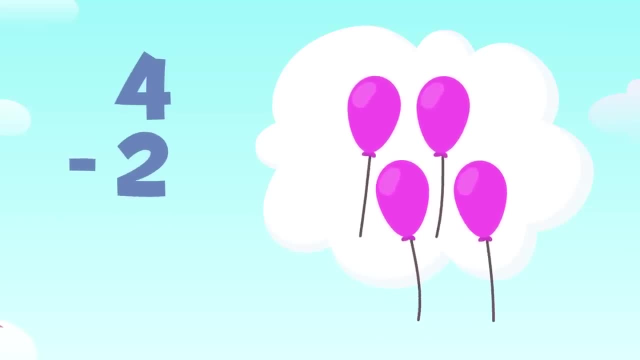 How many balloons will there be left? We need to subtract four minus two. This means that out of four balloons we need to take away two. I'm going to aim well to see how many I'll have left. One and two, Yes. 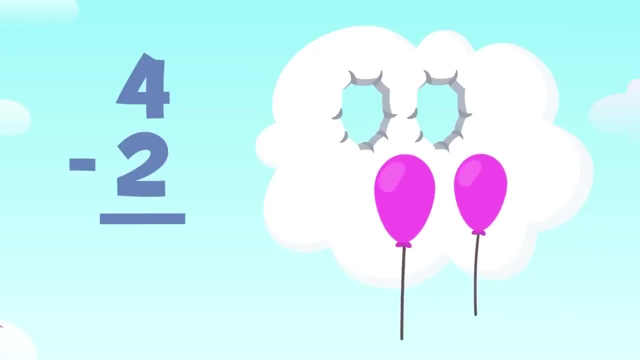 Let's see how many balloons we've got left. One and two. There are two balloons left. The result of subtracting four from two is two. I'm going to aim well to see how many balloons I'll have left. There are two balloons left. The result of subtracting four from two is two. 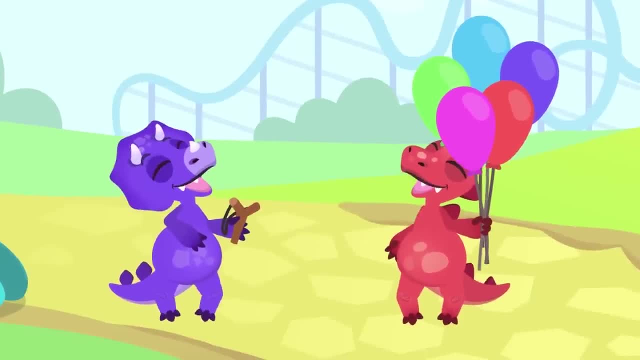 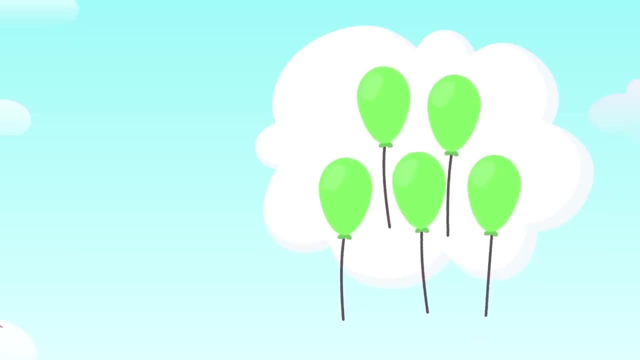 I'm so good at shooting the slingshot, You've let more balloons fly away. There are one, two, three, four and five balloons. How many will there be left if I aim at two of them? The subtraction we need to do is five minus two. 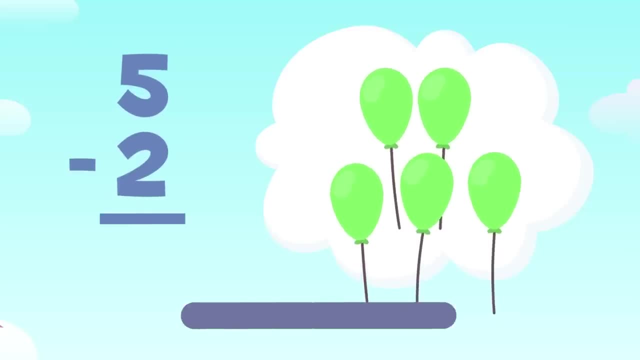 I'll aim at two out of five balloons. What will the result be? One and two- Amazing, Let's see how many we've got left. One, two and three. We've got three balloons left. The result of subtracting five from two is three. 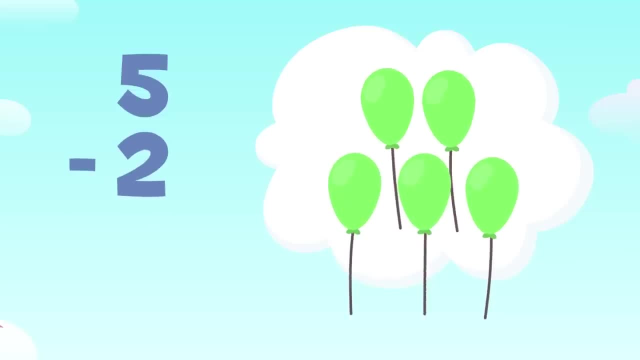 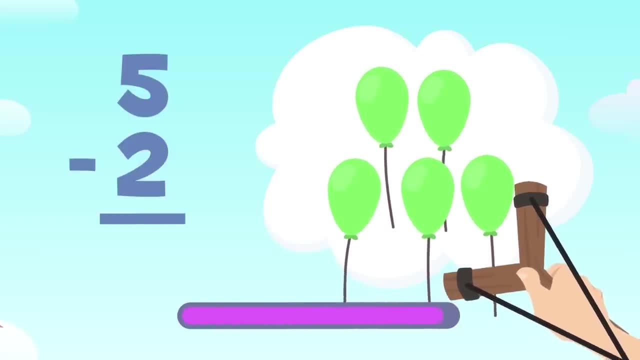 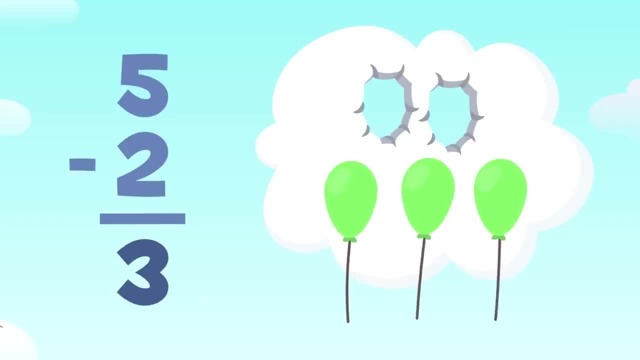 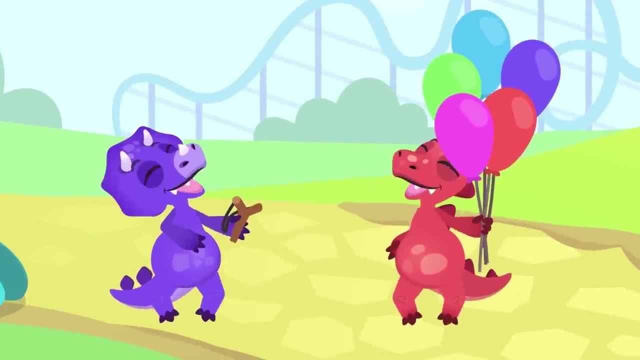 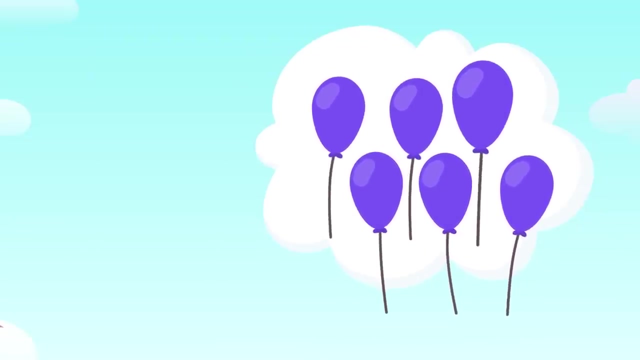 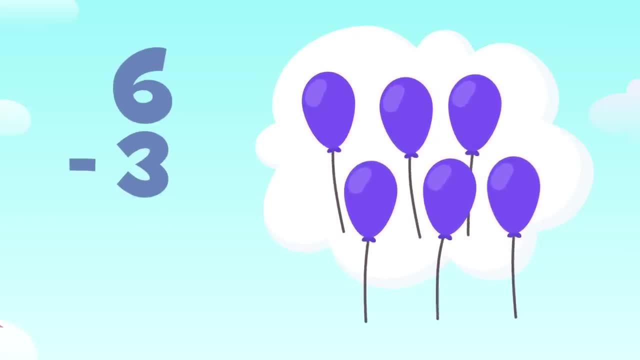 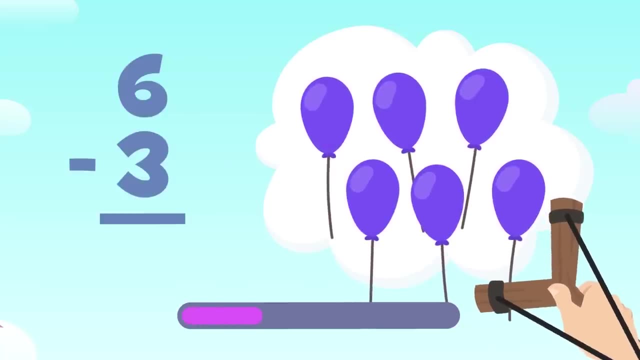 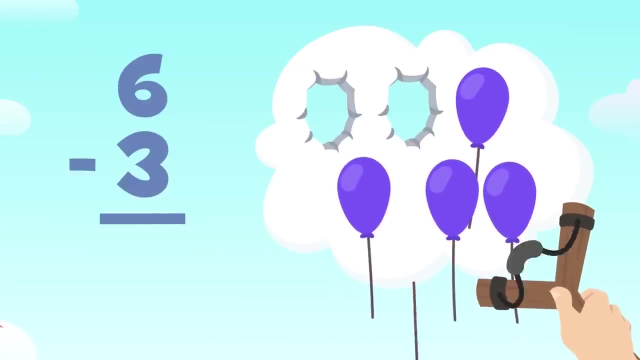 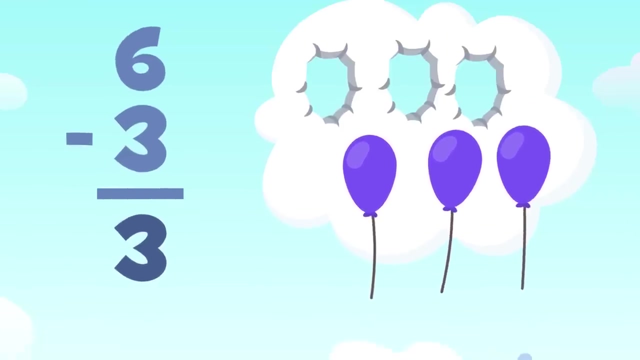 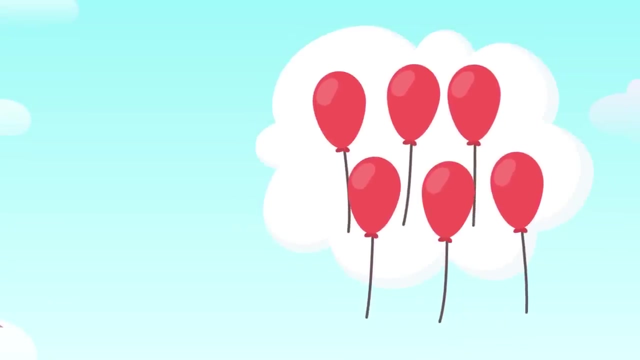 How many will there be if I aim at three of them? what will the result be? one, two and three. yes, let's see how many I've got left. one, two and three. there are three balloons left. six minus three equals three. doing subtractions is great fun. you've let more balloons fly away there. 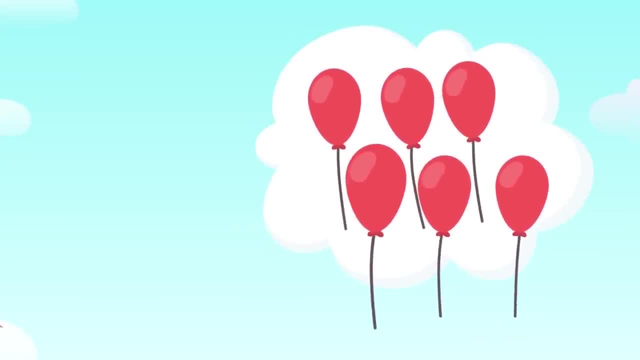 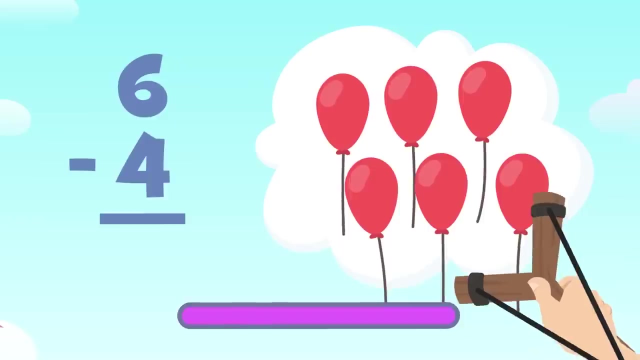 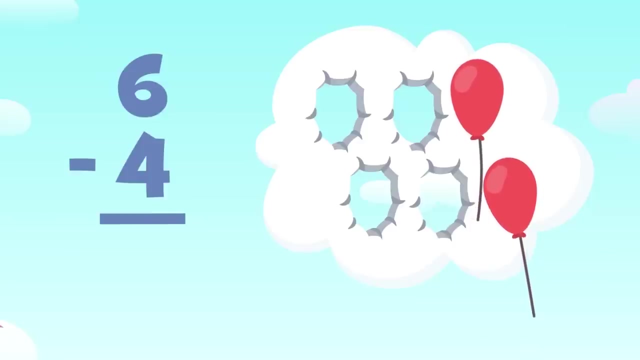 are one, two, three, four, five and six balloons. how many will there be if I aim at four of them? the subtraction we need to do is six minus four. out of six balloons, I'll aim at four. what will the result be? one, two, three and four. swell, let's see how many we've got left. we've got one. 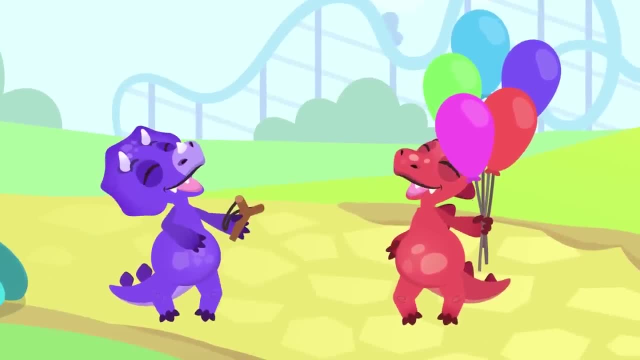 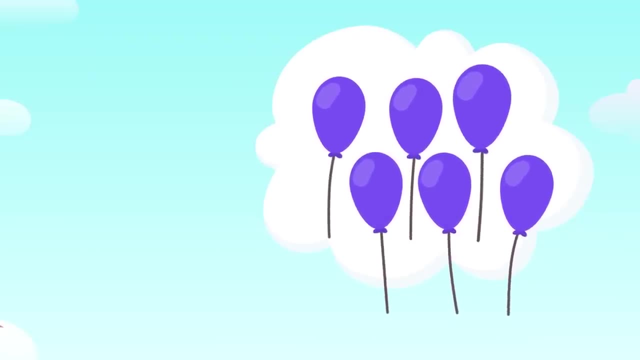 I love playing with my slingshot. You've let more balloons fly away. There are one, two, three, four, five and six balloons. How many will there be if I aim at three of them? The subtraction we need to do is six minus three. 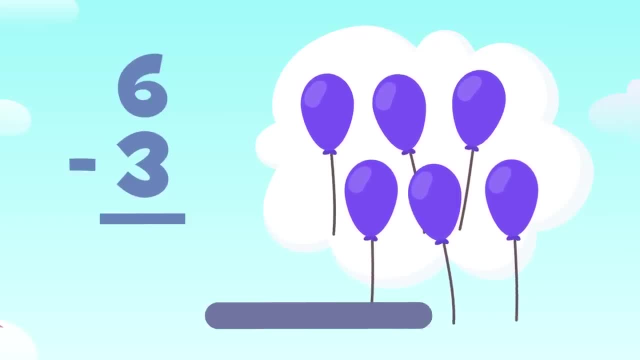 Out of six balloons, I'll aim at three. What will the result be? One, two and three. Yes, Let's see how many I've got left. One, two and three. There are three balloons left. Six minus three equals three. 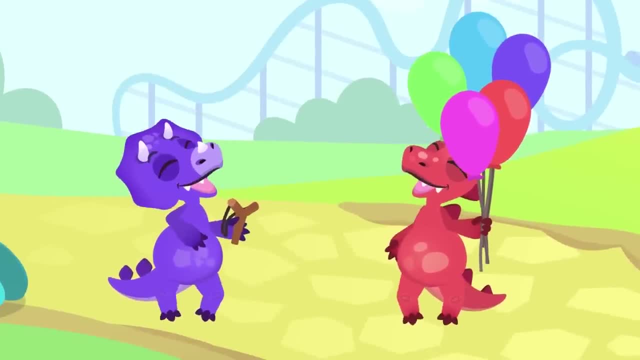 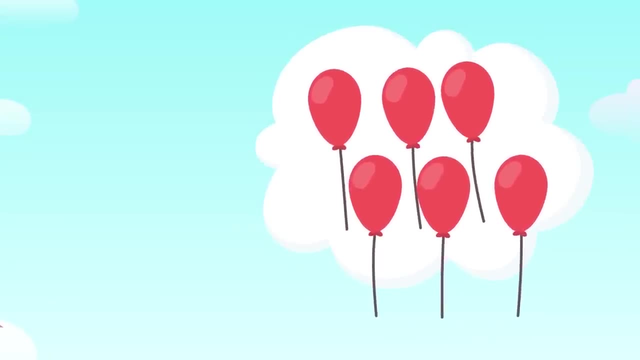 Doing subtractions is great fun. You've let more balloons fly away. There are one, two, three, four, five and six balloons. How many will there be if I aim at four of them? The subtraction we need to do is six minus four. 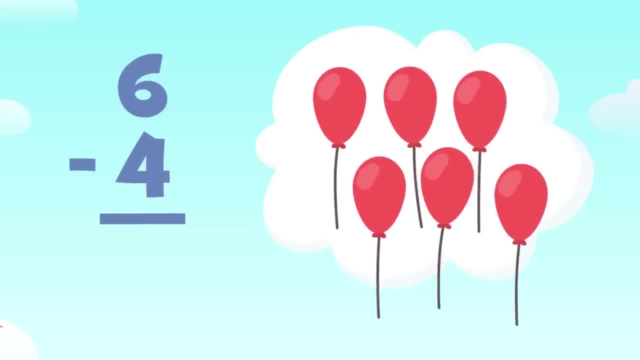 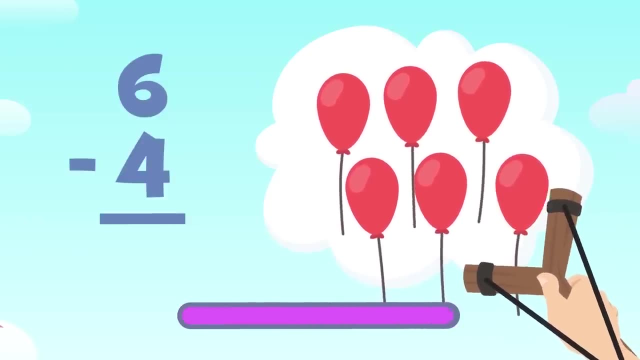 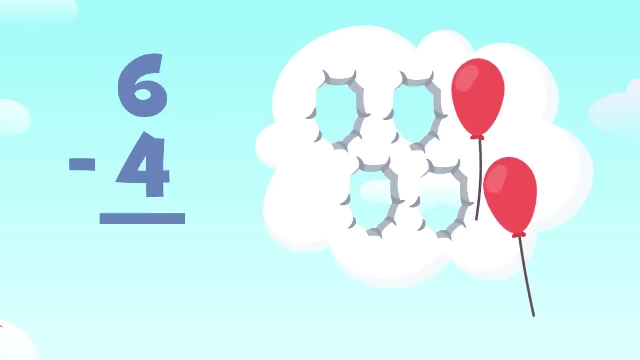 Out of six balloons, I'll aim at four. What will the result be? One, two, three and four. Swell, Let's see how many we've got left. We've got one and two balloons left. Six minus four equals two. 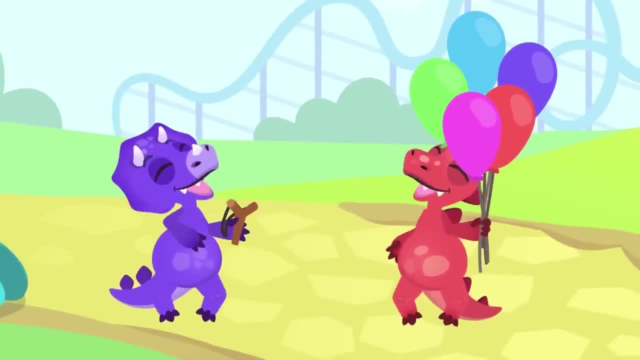 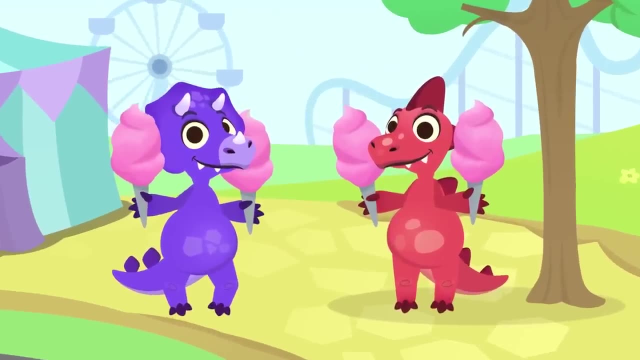 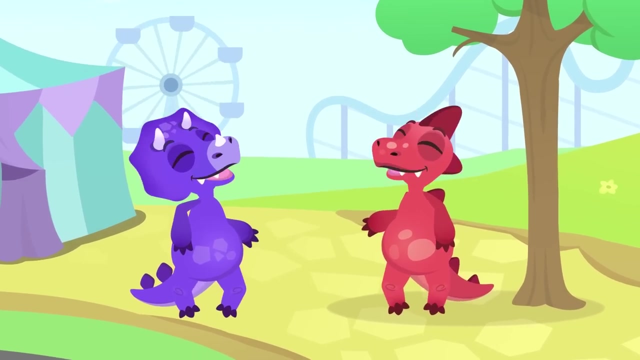 I love doing subtractions. You've run out of balloons, friends. Well, at least you've learned how to do subtractions and you still have all that yummy cotton candy. My, my, you're never full, Oh. 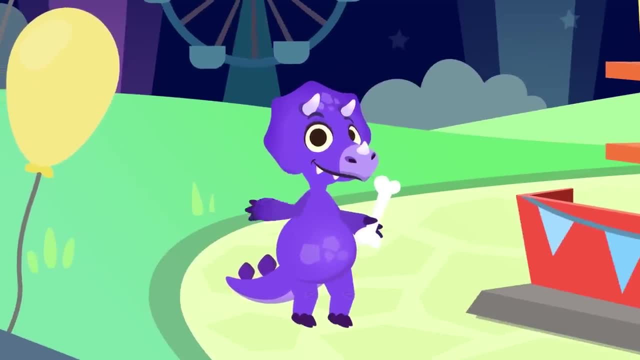 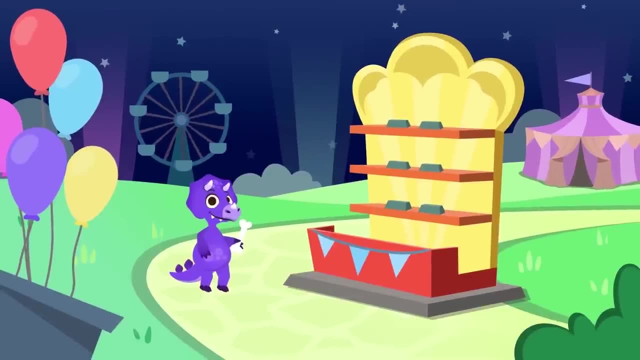 Hi there, Sori, I see you're having a blast. It just occurred to me that this is a great game to practice subtractions. I see you're really good at it. Here's a challenge for you. Are you up for it? 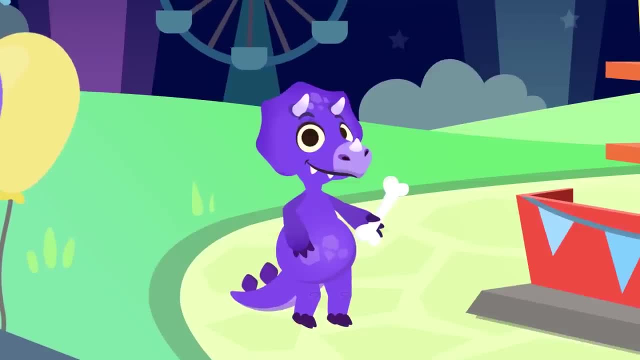 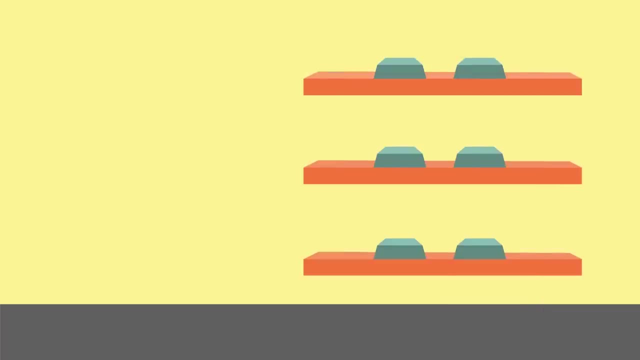 Awesome. This challenge is all about hitting the number of cans. I'll be asking you to, Shall we give it a go. Let's start with something easy to warm up. There are six cans and I want you to hit four of them. 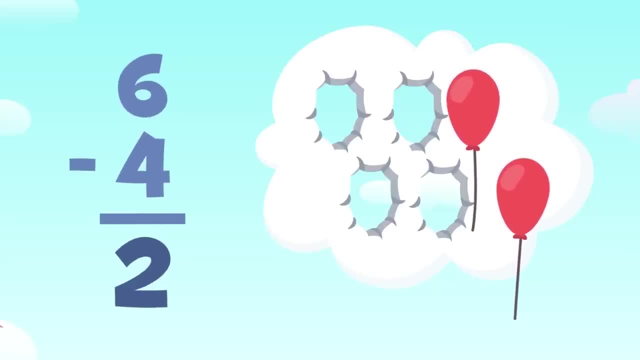 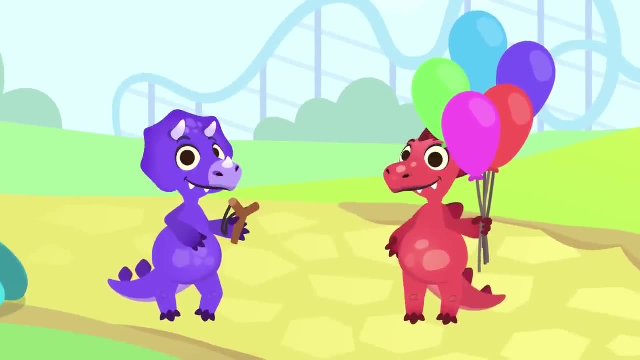 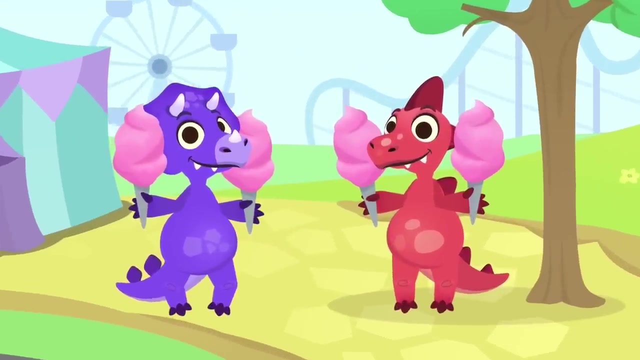 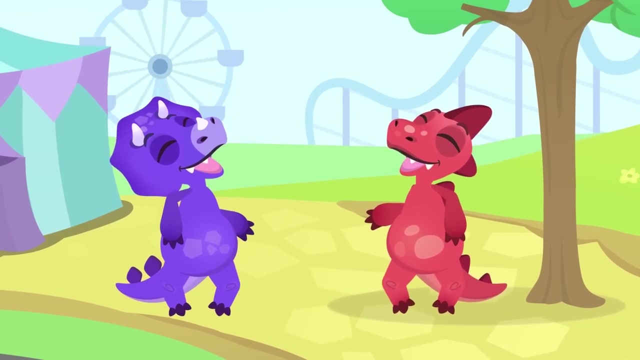 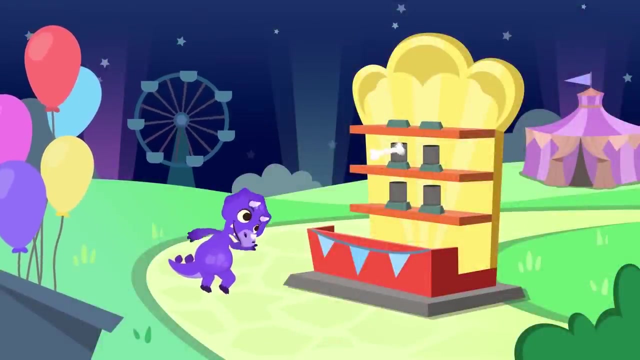 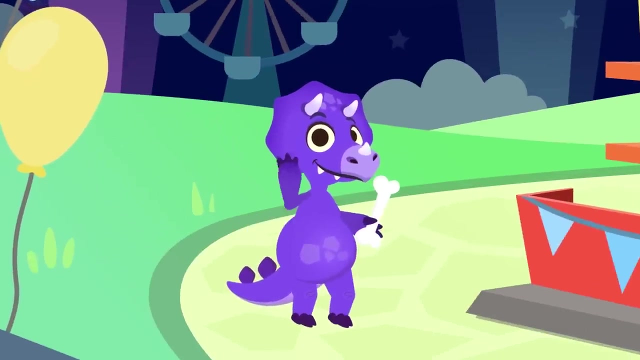 and two balloons left. six minus four equals two. I love doing subtractions. you've run out of balloons, friends. well, let's see how many we've got left. well, at least you've learned how to do subtractions and you still have all that yummy cotton candy. I see you're having a blast. it just occurred to me that this. 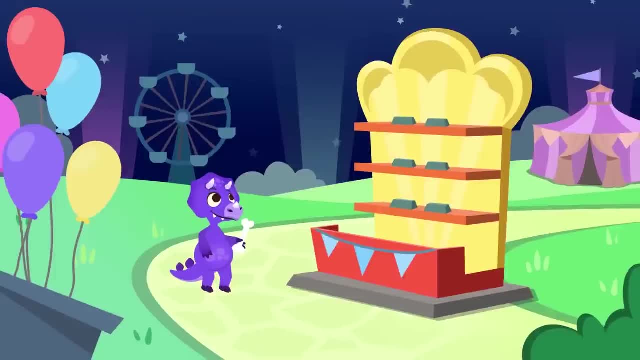 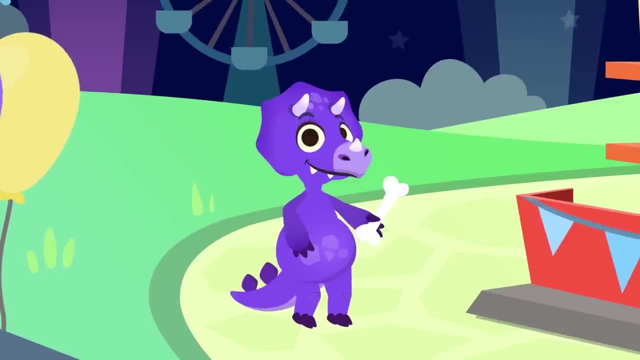 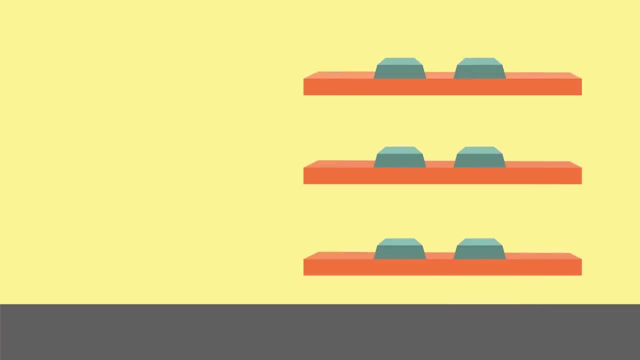 is a great game to practice subtractions. I see your really good at it. here's a challenge for you. are you up for it? awesome, this challenge is all about hitting the number of cans I'll be asking you to. shall we give it a go? let's start with something easy to warm up. there are six. 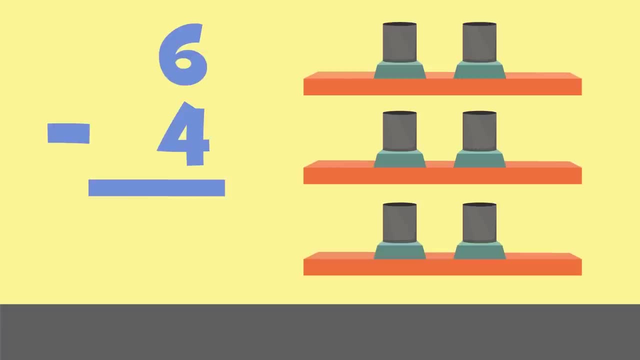 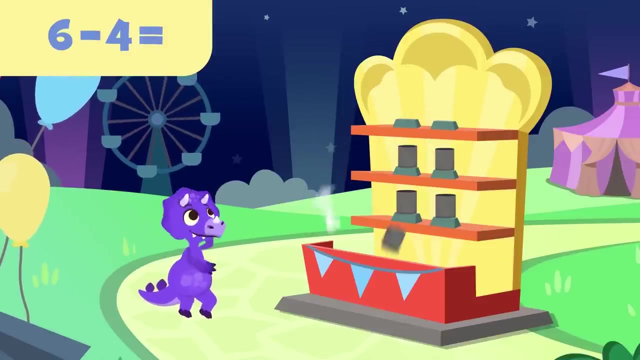 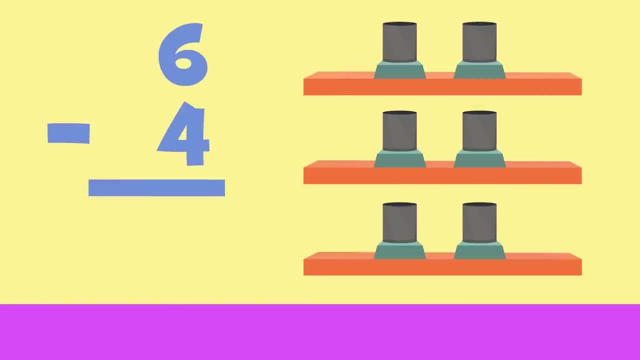 cans and I want you to hit four of them. if you made it, how many cans would there be left time to subtract? you've got it right, go for it. sorry, wait to go. you've hit all four cans. if there were six cans before and sorry, hit four of them now. 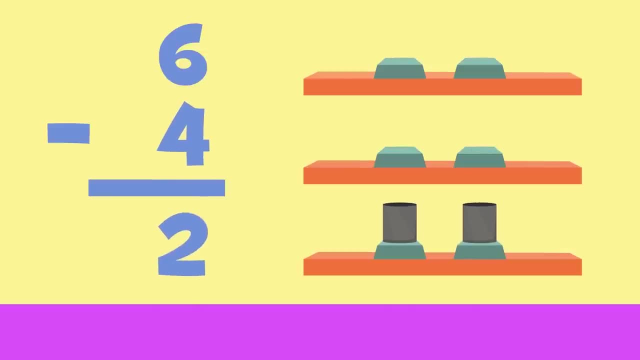 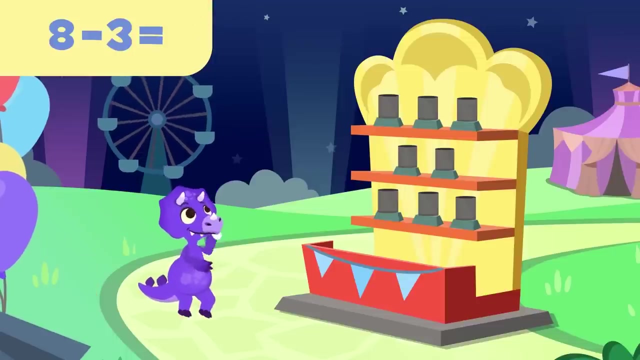 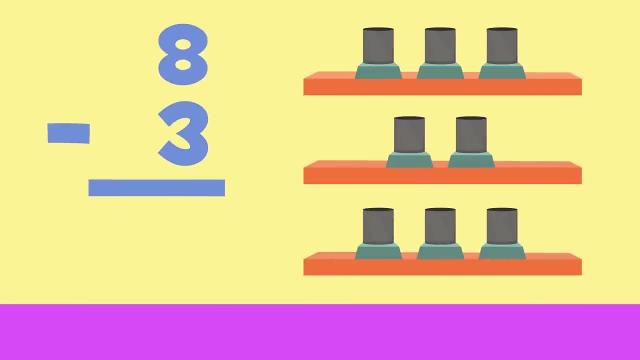 there are one and two cans left. the result of the subtraction problem, six minus four, would be two. let's carry on. there are eight cans. how many will be left if you hit three of them? go ahead and do the subtraction. you've got it right. it's your turn to hit the can. sorry, wow, well done if there. 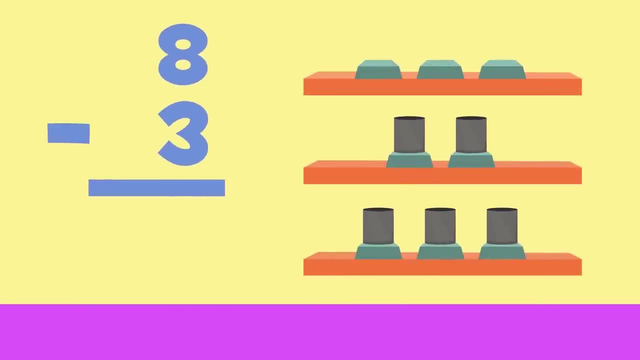 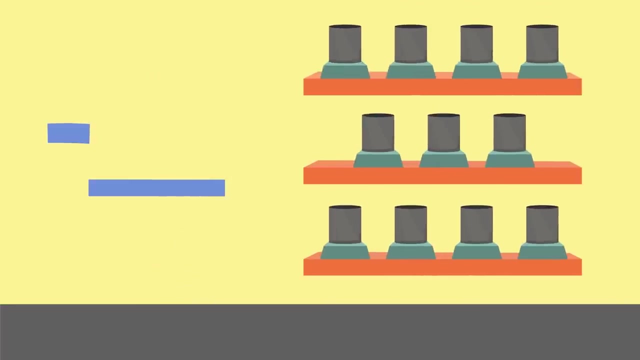 were eight cans before and, sorry, hit three of them. now. there are one and two, three, four and five cans. the result of the subtraction problem, eight minus three, would be five. let's do some more. this will get a little bit more complicated. there are eleven cans now. try to hit five of them. how many will? 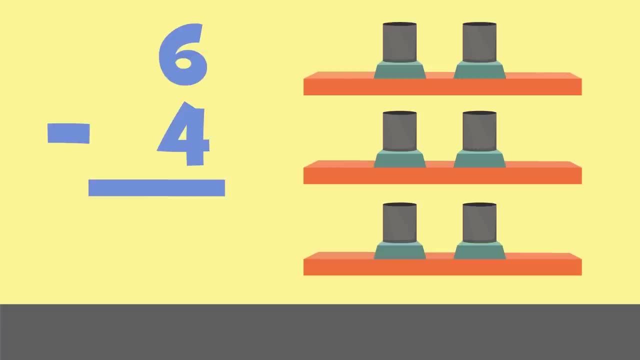 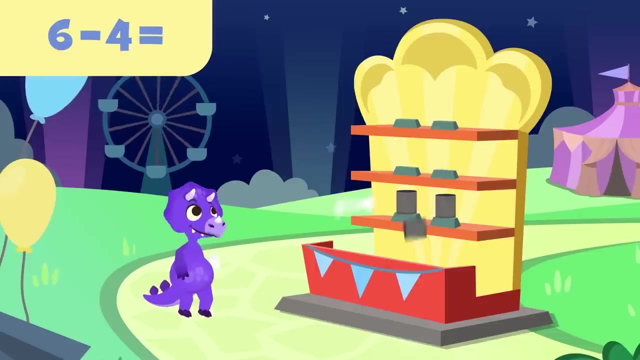 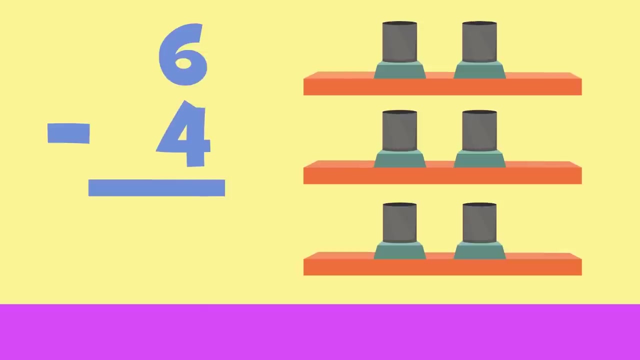 If you made it, how many cans would there be left Time to subtract? You've got it right. Go for it. Sori, Way to go. You've hit all four cans. If there were six cans before and Sori hit four of them, 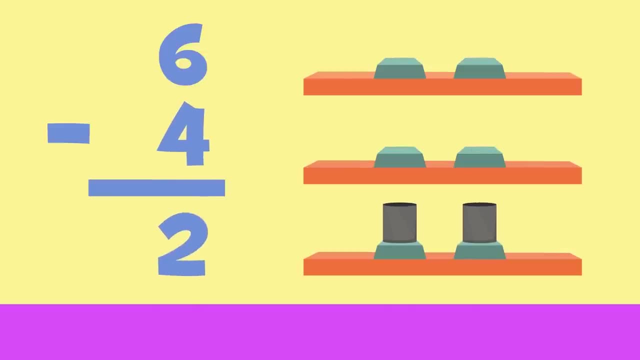 now there are one and two cans left. The result of the subtraction problem six minus four would be two. The result of the subtraction problem six minus four would be two. Let's carry on. There are eight cans. How many will be left if you hit three of them? 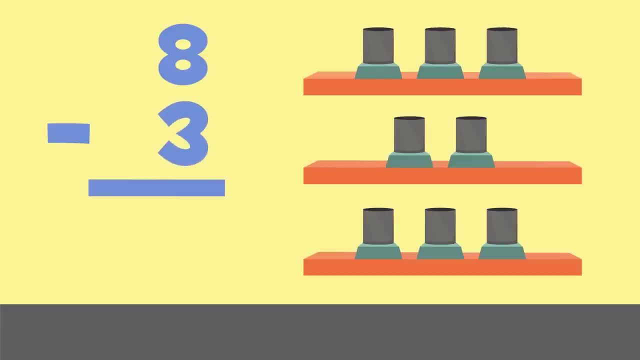 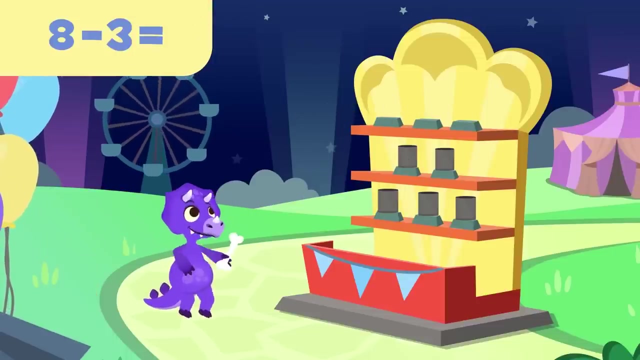 There are eight cans. How many will be left if you hit three of them? Go ahead and do the subtraction. You've got it right. It's your turn to hit the can, Sori. Wow, Well done If there were eight cans before and Sori hit three of them. 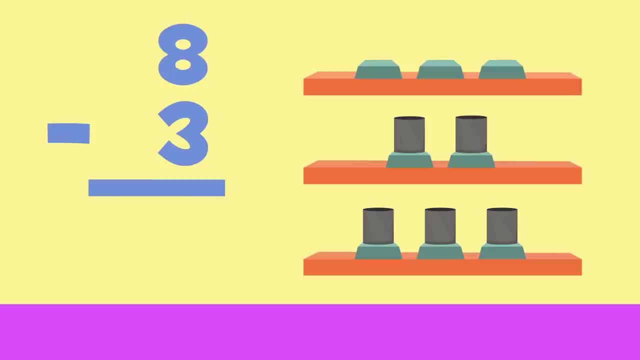 If there were eight cans before and Sori hit three of them Now, there are 1,, 2,, 3,, 4, and 5 cans. The result of the subtraction problem- 8 minus 3, would be 5.. 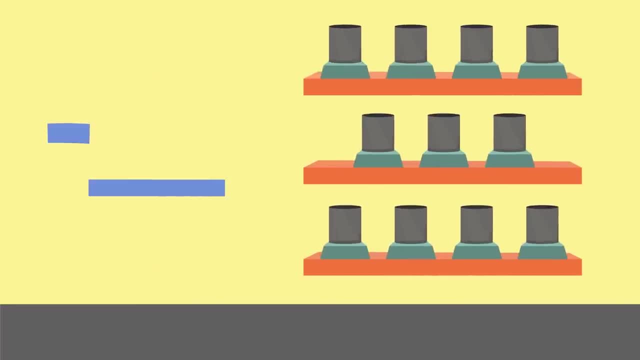 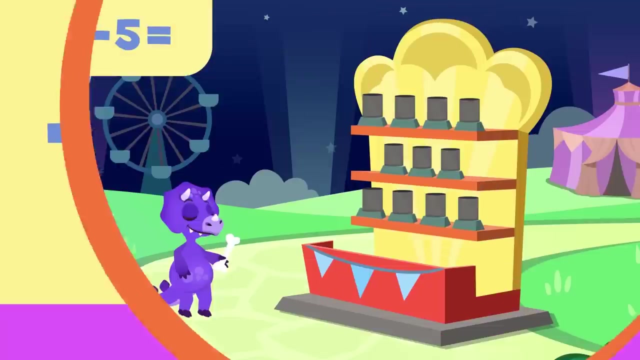 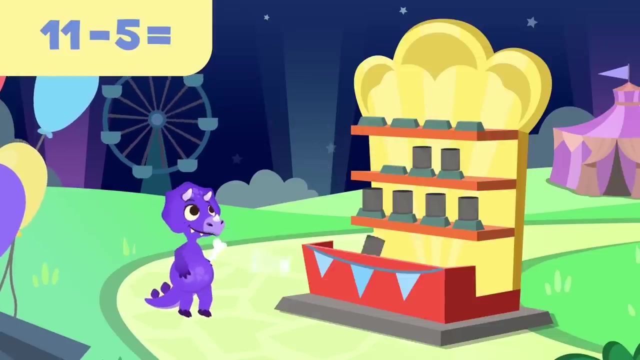 Let's do some more. This will get a little bit more complicated. There are 11 cans now. Try to hit 5 of them. How many will you have left? Let's subtract Ready. Throw that bone, Sori, Nice shot. 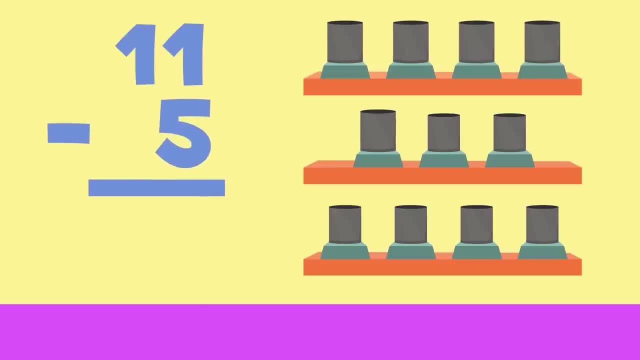 If there were 11 cans before and you hit 5 of them now, there are 1,, 2,, 3,, 4,, 5, and 6 cans left. The result of the subtraction problem- 11 minus 5, would be 6.. 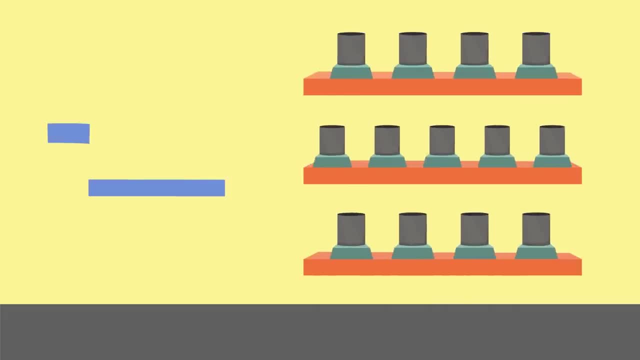 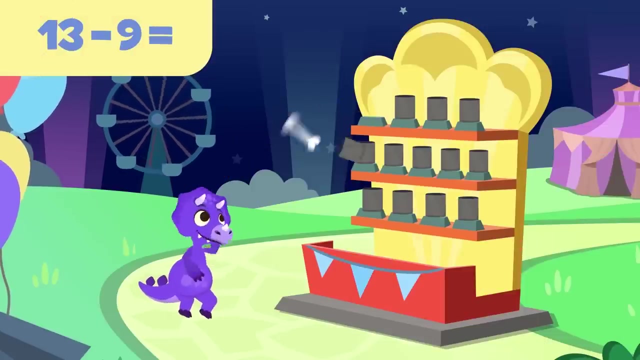 Come on, we're almost there. There are lots of cans- 13 of them. You'll have to hit 9.. Could you Let's subtract Ready? Let's see how good your aim is. Fantastic, You are truly good at this. 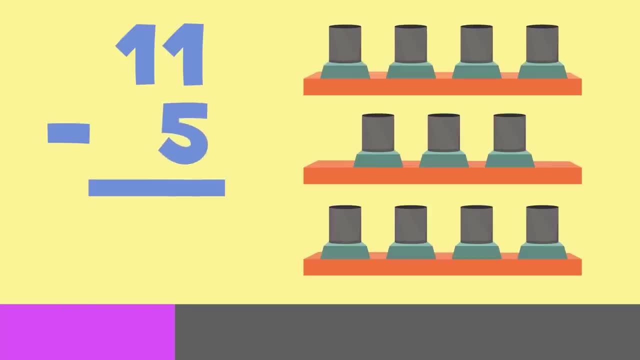 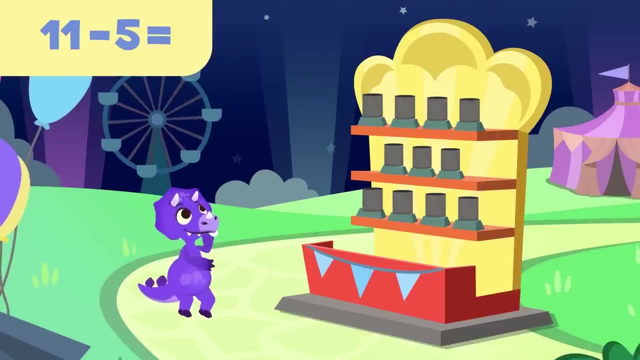 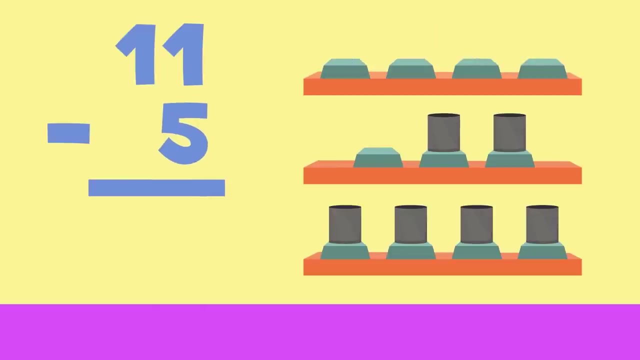 you have left, let's subtract ready, throw that bone. sorry, three. oh, I'm sorry, out of the给 18. can you get there? you're out of the best way. oh, OUR SCART in every gameletHere we go. try more this time, here we go. 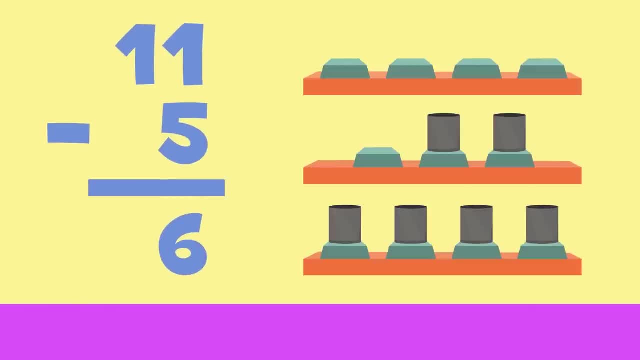 nice shot. if there were eleven cans before and you hit five of them now. there are one, two, three, four, five and six cans left. the result of the subtraction problem, 11 minus five, would be six. come on, we're almost there. there are lots of cans- 13 of them. you'll I'll have to play it all once more. 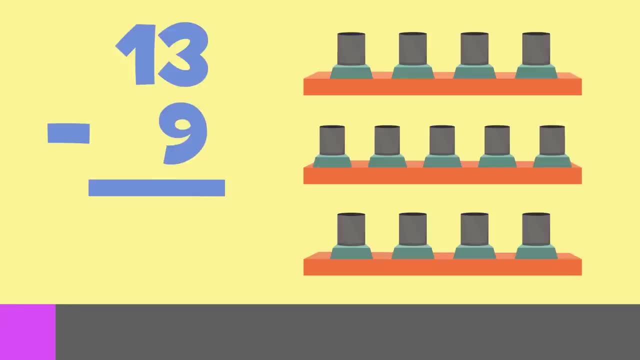 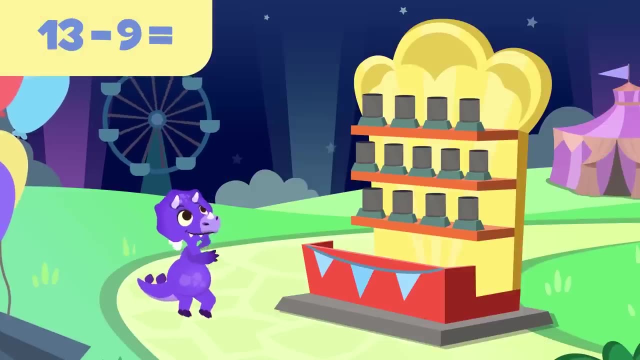 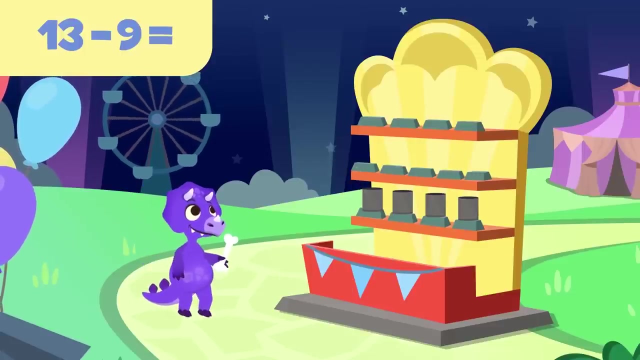 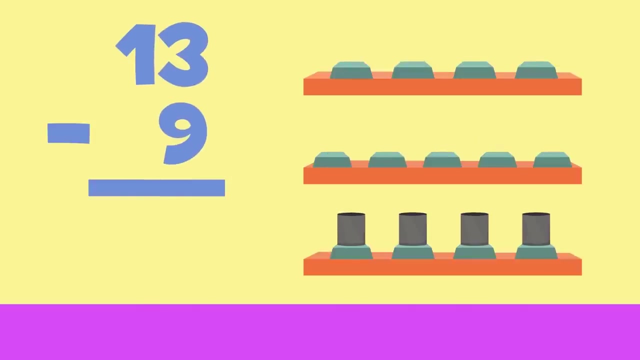 to hit 9.. Could you? Let's subtract Ready. Let's see how good your aim is. Fantastic, You are truly good at this. If there were 13 cans before and you hit 9 of them now, there are 1,, 2,, 3, and 4 cans left. The result of the subtraction problem: 13 minus 9, would. 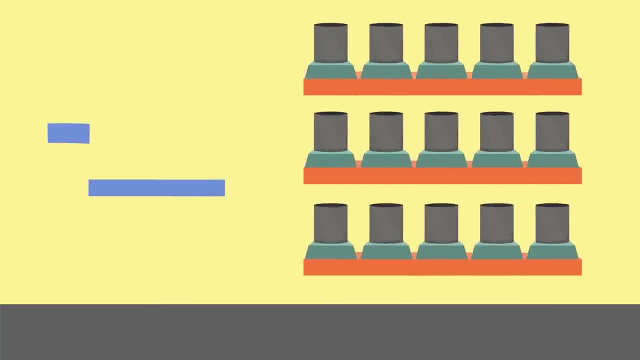 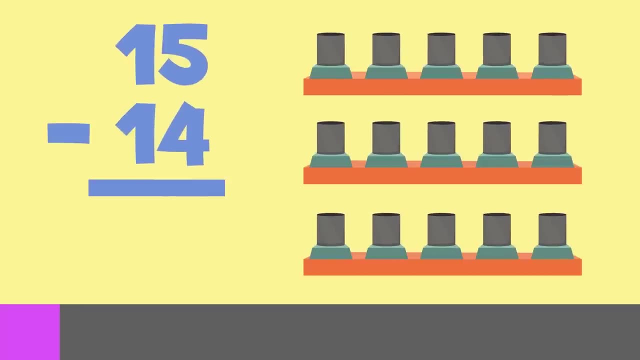 be 4.. Let's do one last try. This won't be an easy one. There are 15 cans. Try to hit 14.. Let's subtract. You've got it right. Last throw. That's a tough challenge. 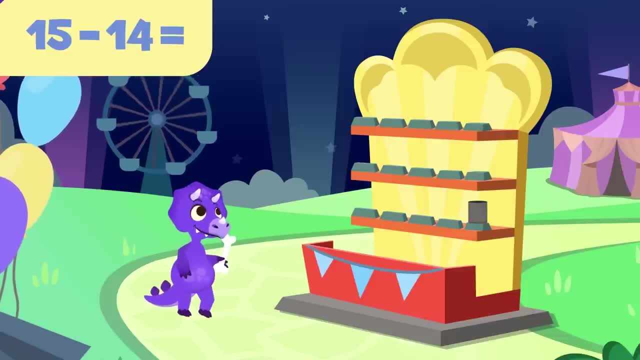 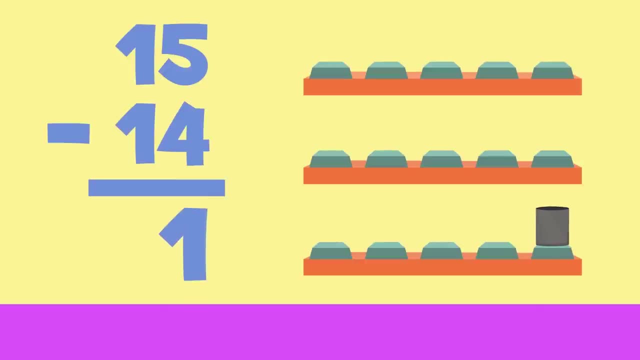 Incredible. You're such an expert. Sori, If there were 15 cans before and you hit 9 of them now, there are 15 cans left. The result of the subtraction problem- 15 minus 14, is 1.. Your aim is awesome, Sori, You've. 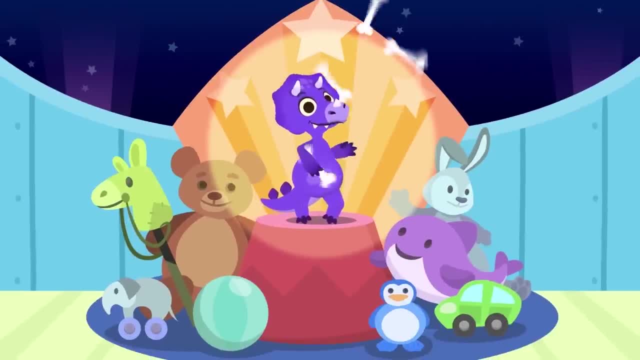 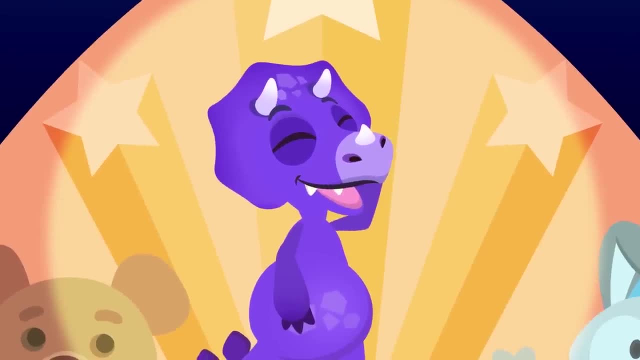 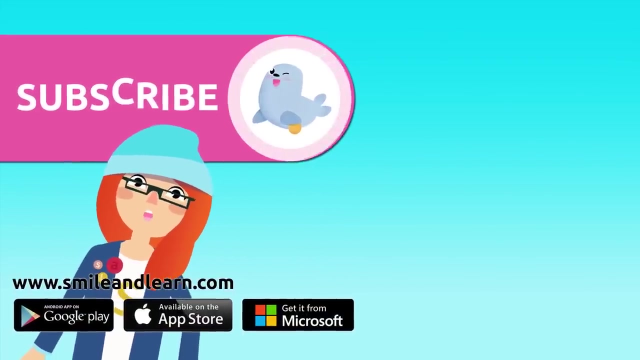 won so many prizes. Sori, Congratulations. Subtracting is great fun Ouch. That must have hurt. Ha ha, ha, ha ha. Did you like the video? We have so many more. Subscribe by clicking on the seal: Ah and. if you want to keep watching more videos, click on the boxes.